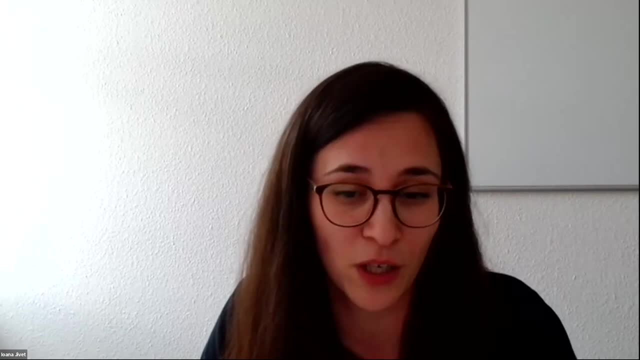 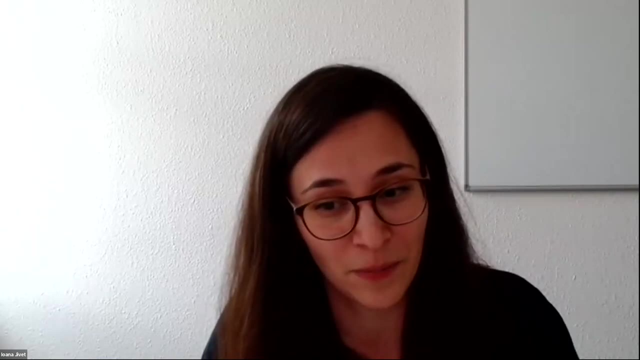 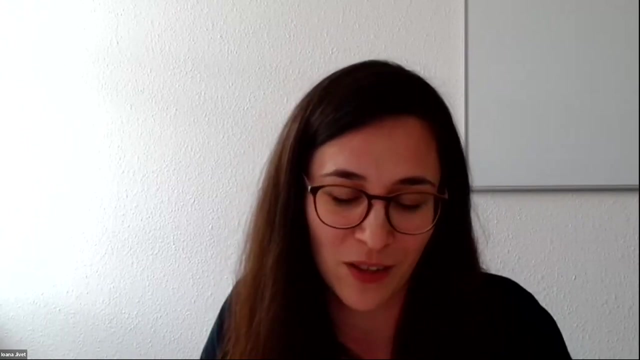 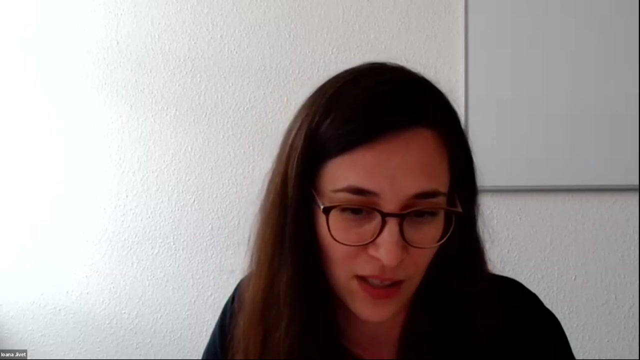 She's also an affiliate of the Center for Change and Complexity in Learning at the University of South Australia In Munich. she leads the LiEBS research group that studies learning analytics and practices in systems, and her current research focuses on creating impactful technology based interventions that use learning analytics and support agency and social networks in higher education and workplace training. 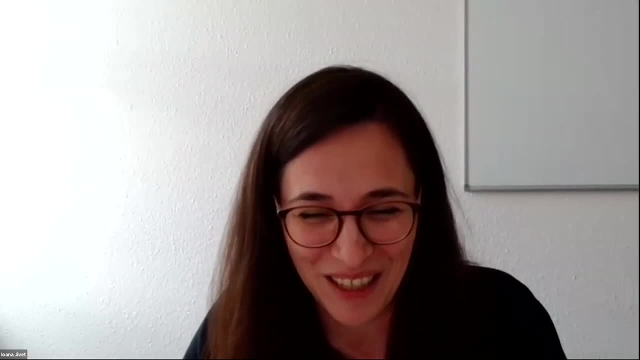 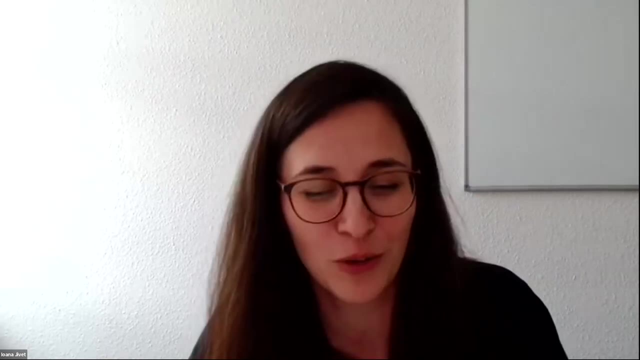 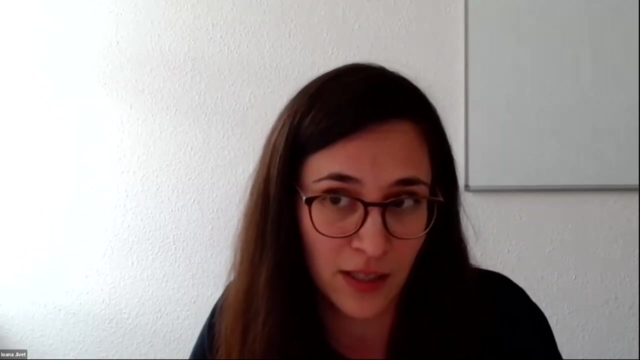 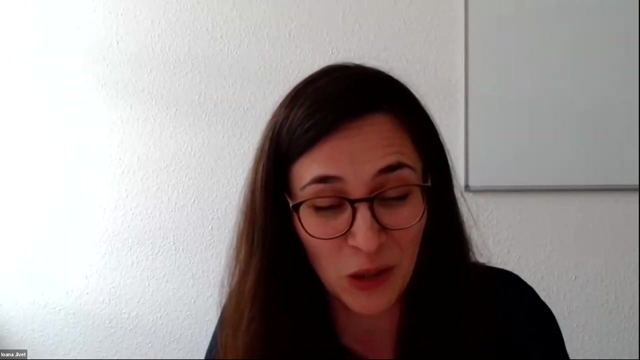 The topic of today's talk is this: Today's work seminar is theoretical underpinnings and methodological toolkits and a methodological toolkit of complex dynamical systems, and our speakers will highlight their relevance to, and potential integration with, learning analytics. Thank you for being here today and sharing your research with us. 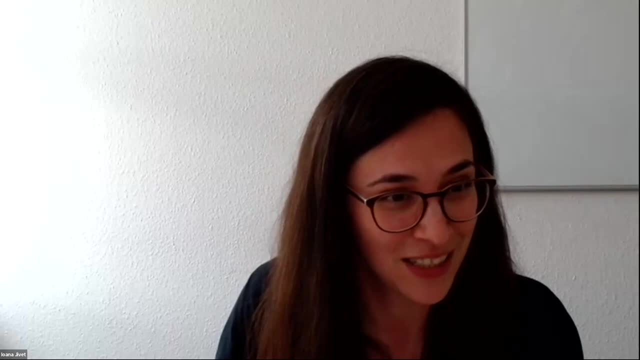 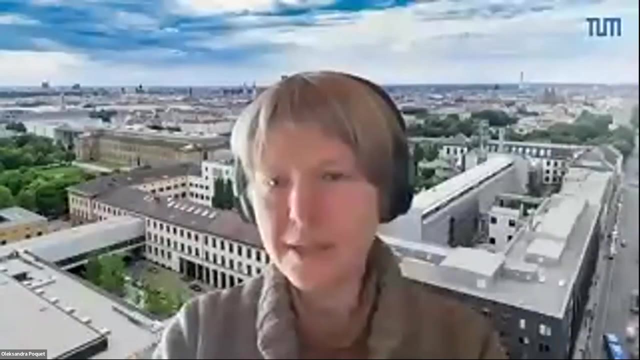 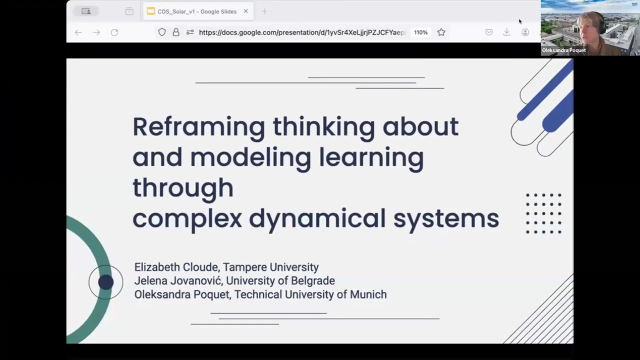 I now give the floor to you, Sasha. you will be sharing your screen first. Yes, thank you so much, Ioana, for the introduction. Please allow me a moment to set the right screen in motion And you should see my screen. 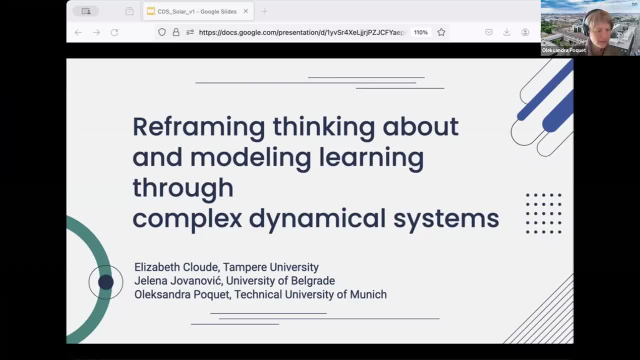 Okay, And just bear with me another second and we can start. So, okay, well, wonderful to see you all. Thank you for the introduction and it's an honor for us to be here and we want to thank you. Thank you, Soler, for inviting us to talk about complex, dynamical systems and learning. 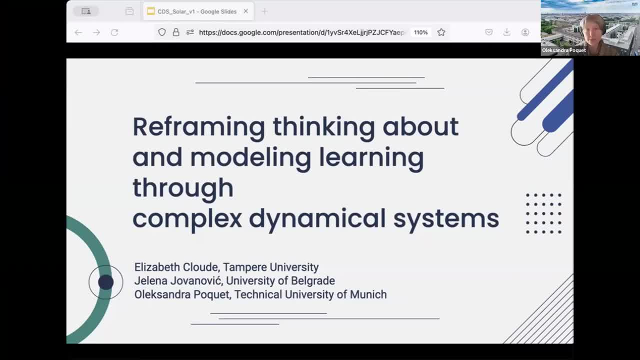 analytics. My name is Alexandra or Sasha and I'm a professor at the Technical University of Munich doing this talk together with two of my colleagues. I'm just going to ask them to wave their hands because they talk later. Sol is cloud. just then was Jelena Jovanovic. 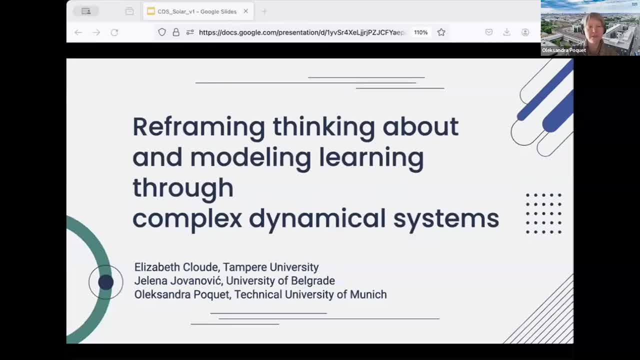 Thank you very much to you both. So before we start- and I'd like to start, given that time is running for us- we want to say that the arguments about the relevance of complex dynamical systems to learning sciences are not new, and are not new to us for sure. 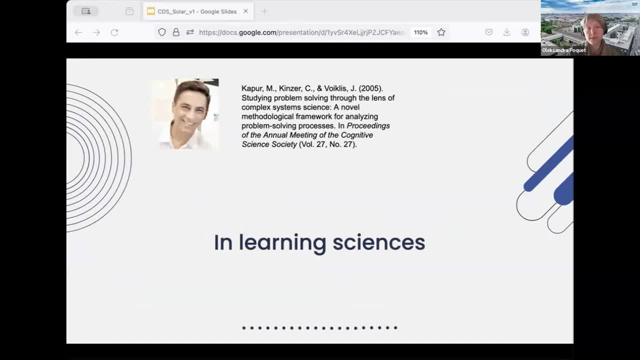 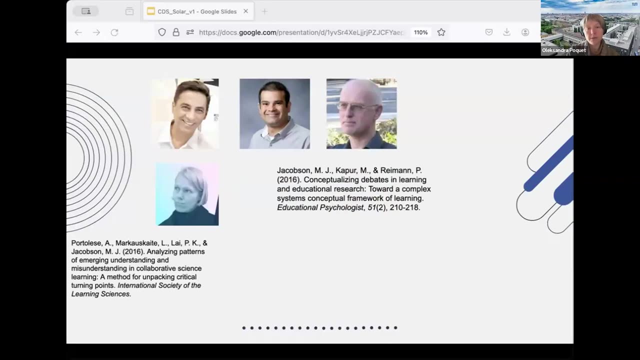 Kapoor's work is a stellar example of integrating complex systems into the analysis of learning. DeMello's research has had consistent flavor of complex, dynamical systems thinking. Jacobson Ryman and Marcos Keiter offer ways of seeing complex systems as a meta-theory. 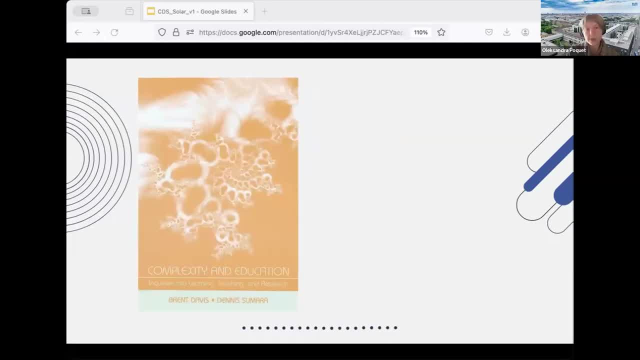 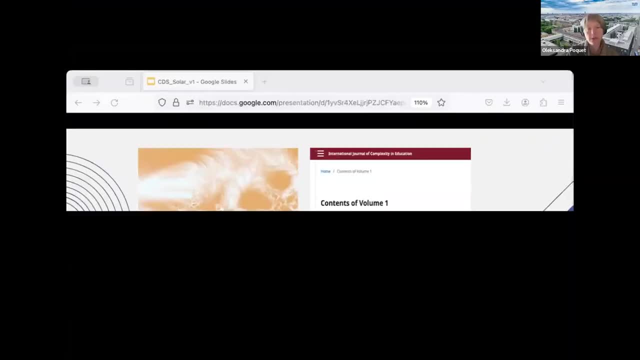 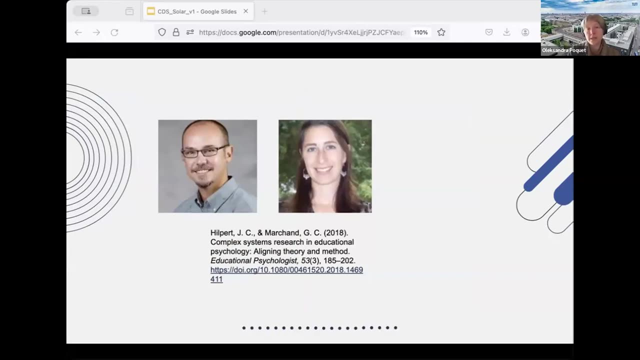 over the cognitive and situated divide. Davis and Sumatra summarized some of this thinking in their 2006 book, and important work has been put in place. Important work has been published in the International Journal of Complexity in Education. We must mention in this intro an excellent piece by Hilbert and Marchand that summarizes: 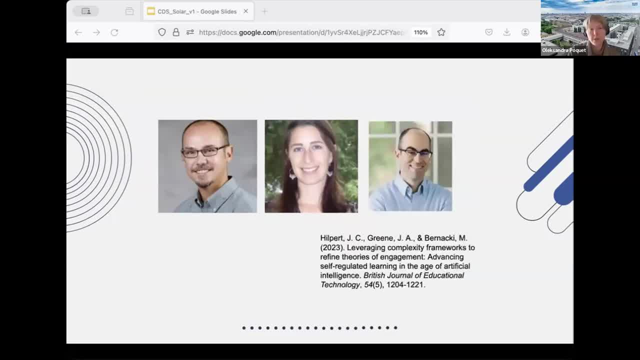 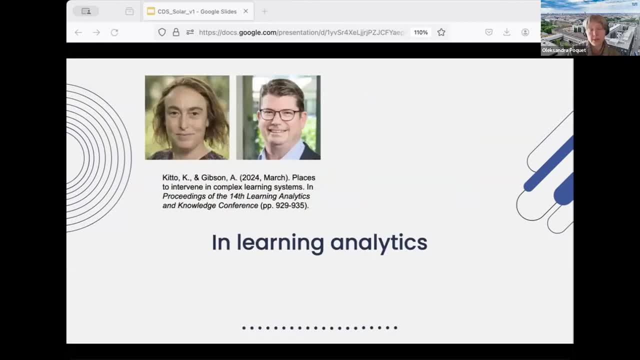 principles of CDS for educational psychology and recent work on this by Hilbert Bernanke and Green. We also must talk about people whose research relates to complex systems in learning, analytics, such as Kitto and Gibson with their latest log paper on interventions Dinder and Cloud. 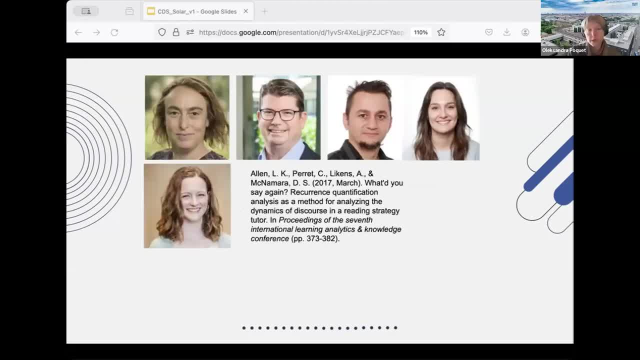 with work on effect and collaborative groups. Alice please, Paule, Deva, Whitebuch and Azevedo with work in self-regulated learning. Lopez, Pernas, Sackler and Nixon with modeling collaborations in complex systems. 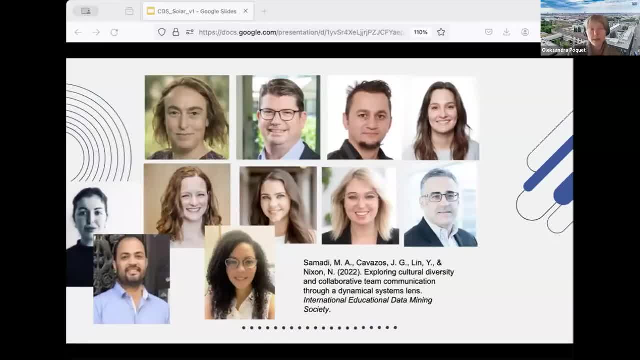 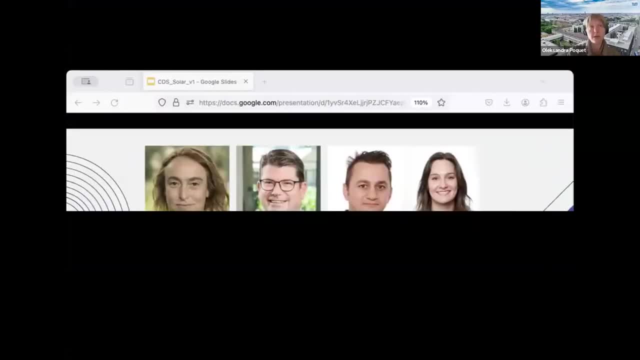 David Whitebuch and Azevedo, who work on self-regulated learning, Lopez, Pernas Sackler, with ideological approaches in learning analytics. Now, this is not an exhaustive list, of course, of people who are looking at how to integrate. 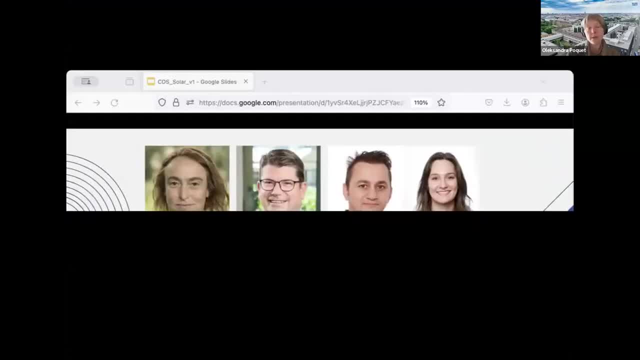 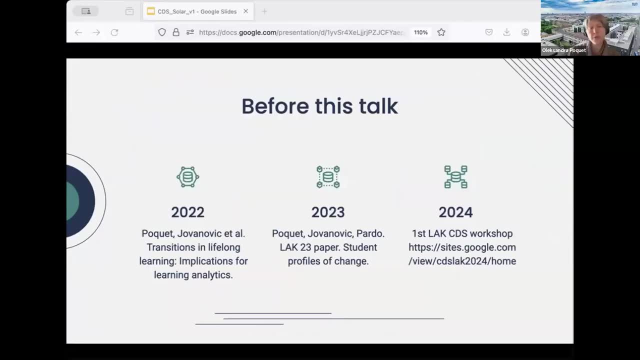 complex systems in learning analytics or learning sciences. But at least here the hope is to demonstrate that pockets of complex systems work have existed for a while Now. for the three of us, the three of us. what brings us here is the fascination with these ideas. So we wrote some. 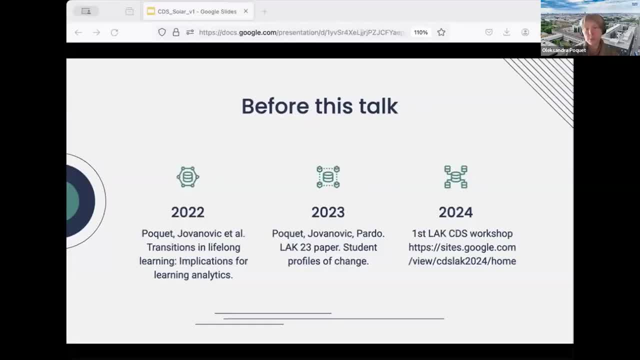 papers on this, one of them being the best paper at LAC last year, which is why we were invited to talk about it, Thank you. And also more recent work last March, past month, where we had the first workshop on complex dynamical systems and learning analytics that we organized. 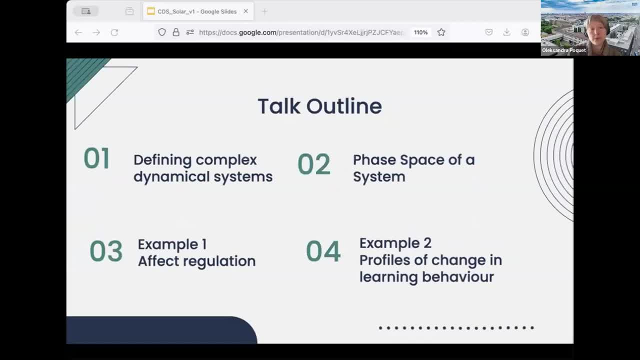 Now, moving to the talk. today we will offer only one possible definition of a complex, dynamical system, to try and bring everybody on board with one example, And then I will explain just one theoretical idea from complex systems and that of a phase space to scaffold your understanding. 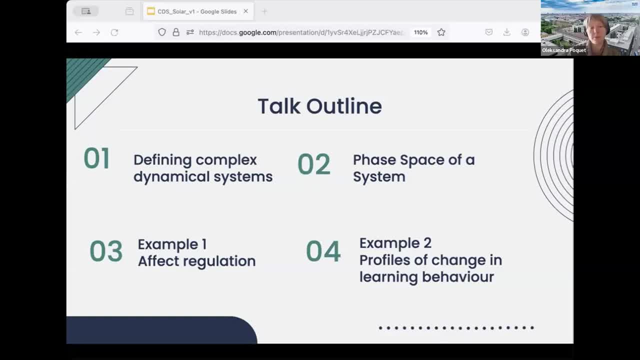 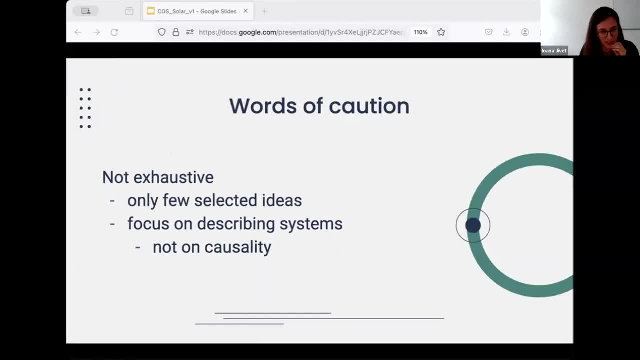 of the two examples of how these ideas can be used that Yelena and Liz will present to you, And I also want to say a few words. I'm sorry, The screen is flickering for us and it doesn't seem to be stopping. Would you just stop and share? 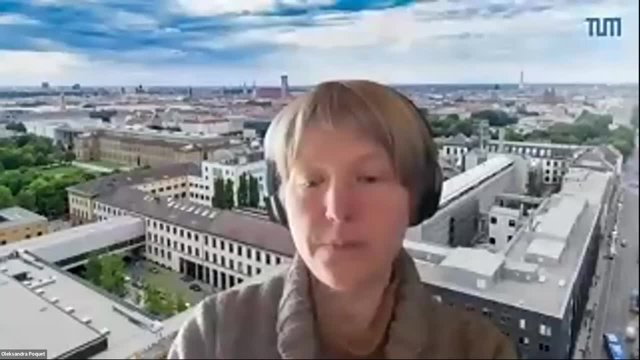 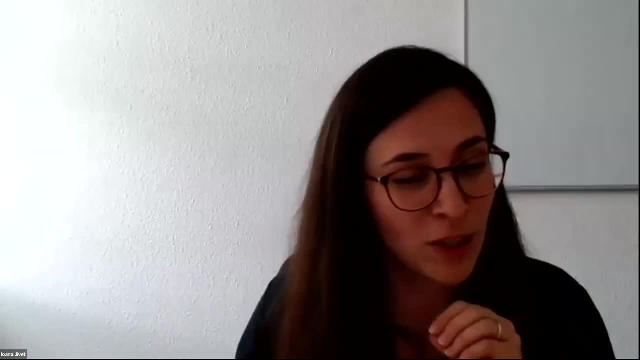 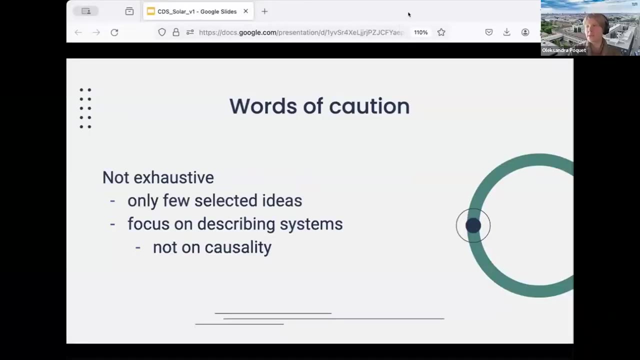 the screen again? Yep, absolutely, Absolutely. How early did you lose me? No, no, we heard everything. It's just that the screen is flickering, Everything is just. How is this? No, I think it's still flickering, But I'm not sure why. 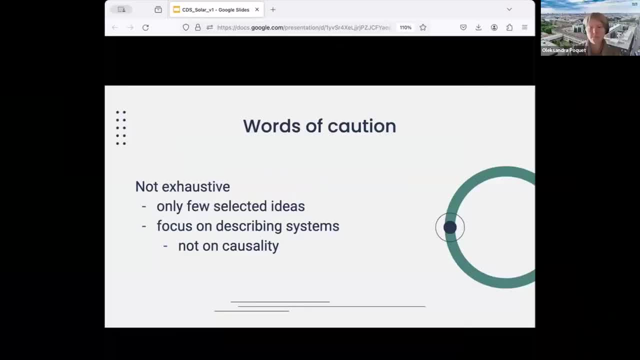 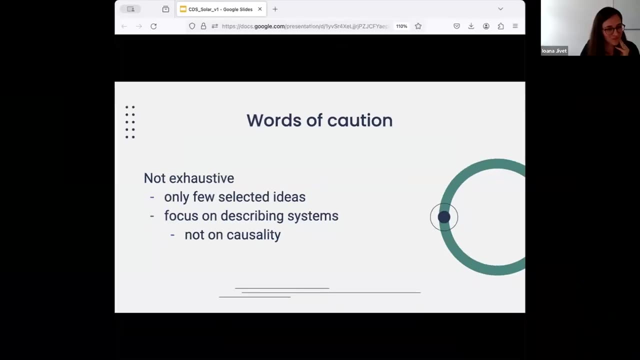 But I guess, yeah, we'll have to continue like this for now. I think Now it's Well, the only Is it okay, All right, So let's use this and see how this goes. Please stop me if this is not making sense. 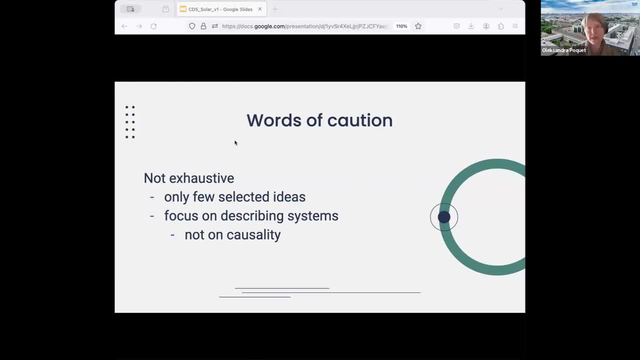 So, to go back to what I was saying was that there's a huge body of, There's a huge body of work, actually both theoretical and methodological, in complex systems, research in relation to learning, and we will only pick one idea that we'll try to unpack and exemplify for you. 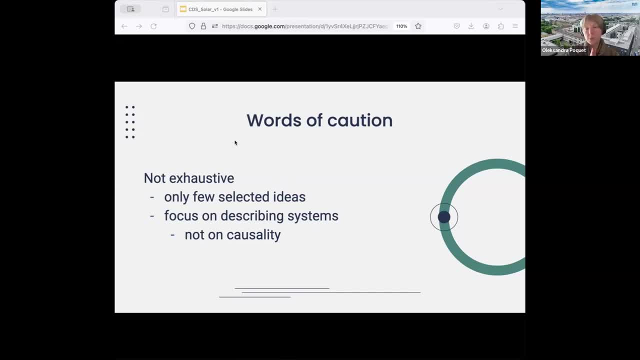 But, importantly, this is just one idea and the range of other, both theoretical and methodological application is much broader than what we'll talk about. and also we will not talk about causality, because causality has a very special understanding in complex systems. 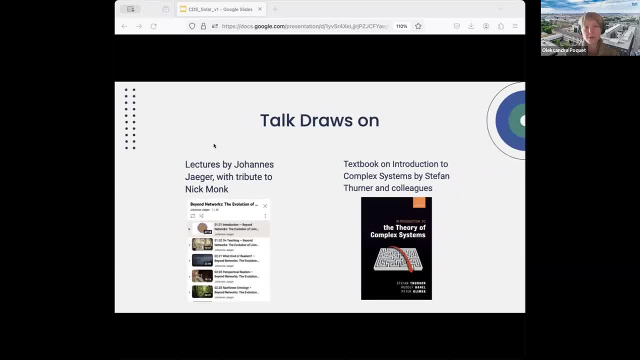 Okay, So let's move on to the next slide, hopefully, and some words of credit. So I will. I want to acknowledge some of the resources that we used in being inspired of how to explain this better, And so the explanations stem from the work by Johannes Jäger and Thörner and colleagues. 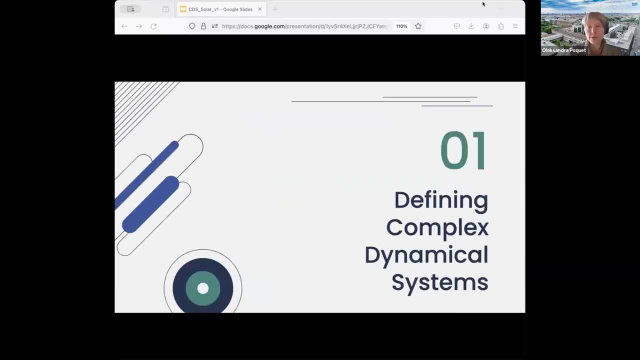 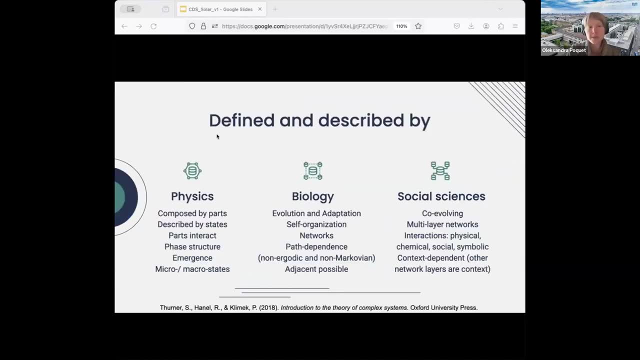 So now, moving on to the content of the talk, How do we define a complex, dynamical system? Complex systems theory itself is an evolving area of science and the description of complex systems come from physics and biology and social sciences. And you can see some words here in the slide, but this is just to show a range of theoretical complexity that exists. 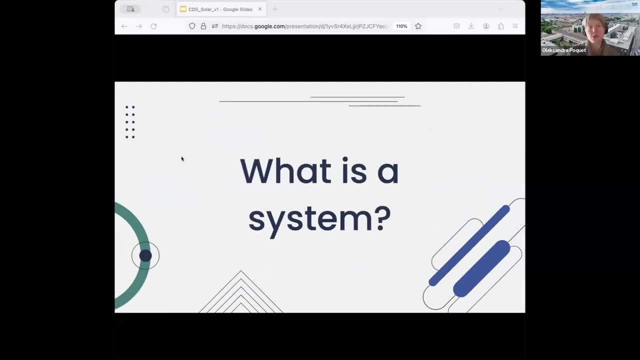 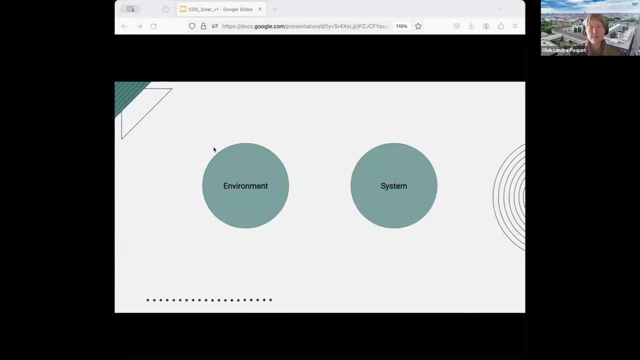 And, of course, because of that, the definitions that exist as to what a system is are many, But I think the useful one is starting from the point that defining a system, that is, a part that comprises of components That interact and produce some properties, is defining a system in setting it apart from its environment. 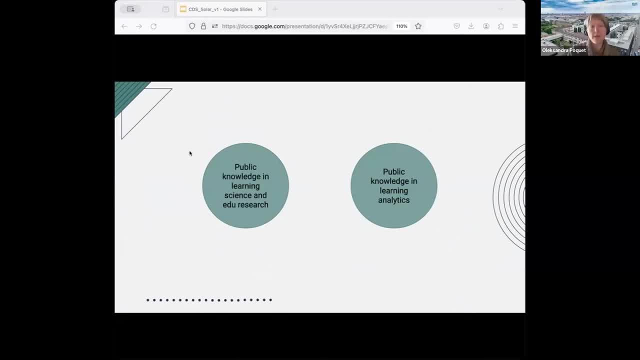 So the example, a toy example here. let's imagine that all public knowledge and learning analytics can be viewed as a system. So that's the system on the right and we are separating it by defining it that way from the environment. So the public knowledge in learning science and education research on the left. 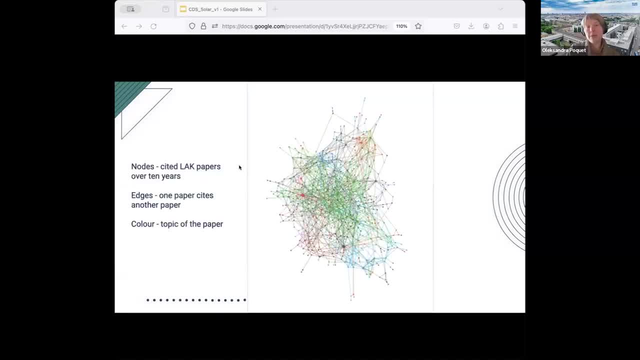 The system of public knowledge in learning analytics can be represented as a network, And I work a lot with networks, So here's my name. This is a network slide here. This is a system where you see each note is paper. in luck, Color is the topic of the paper. 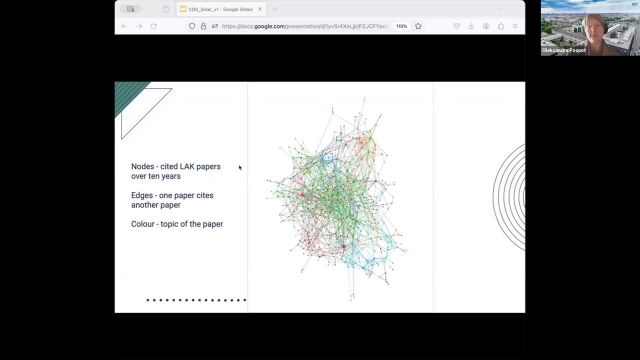 Connections are how these papers cite each other. We can say that this is a system of knowledge publicly available and sort of prominent themes in this domain. We can describe this system at the macro level by saying there are emergent themes and trends and sort of important methodological considerations. 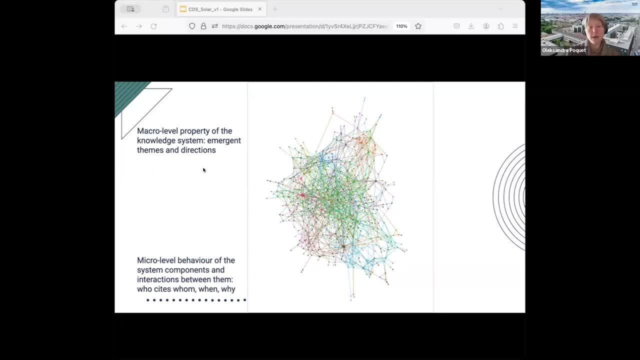 We can also describe this system at the micro level By looking at how individual papers cite each other, in which section, by which authors, at which point in time, et cetera, et cetera. And we also know from complex systems theory that micro level processes. so these micro level work drives what we observe at a macro level of the system. 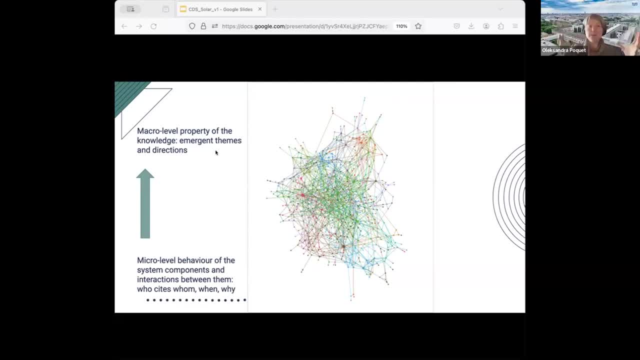 And that once the macro level sets, so, for instance, once we have themes and rules of what sort of is acceptable within this public space, And that once the macro level sets, so for instance, once we have themes and rules of what sort of is acceptable within this public space, And that once the macro level sets- so, for instance, once we have themes and rules of what sort of is acceptable within this public space- Then the micro level behavior will be constrained by the macro level process. Then the micro level behavior will be constrained by the macro level process. Then the micro level behavior will be constrained by the macro level process. And we also know from complex systems theory that these kind of systems, they have feedback loops that take place between the different components of the system as this sort of system develops. And we also know from complex systems theory that these kind of systems, they have feedback loops that take place between the different components of the system as this sort of system develops. 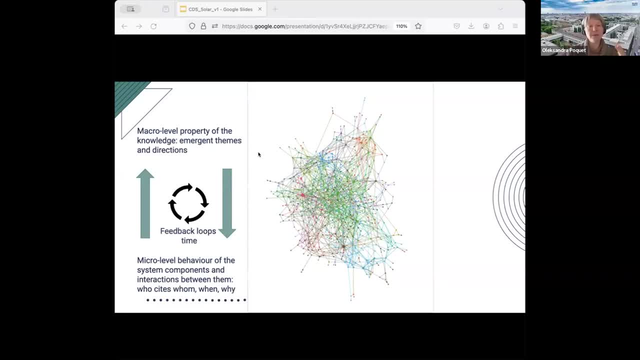 And we also know from complex systems theory that these kind of systems they have feedback loops that take place between the different components of the system. as this sort of system develops theory that these kind of systems, they have feedback loops that take place between the 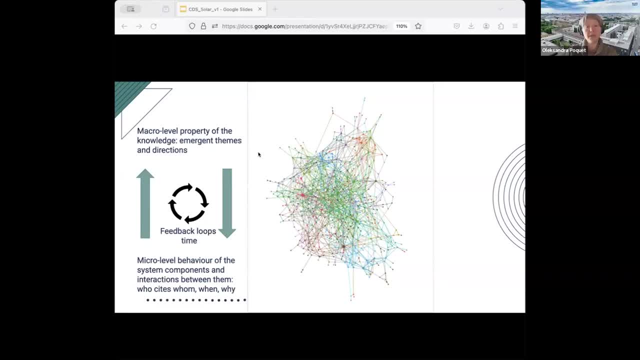 different components of the system as this sort of system develops, in this case, as the scientific discourse evolves. Now, if you were listening to me, you probably heard that there is a little bit of a discrepancy between what I say and what I show. My language has a lot of the movement and 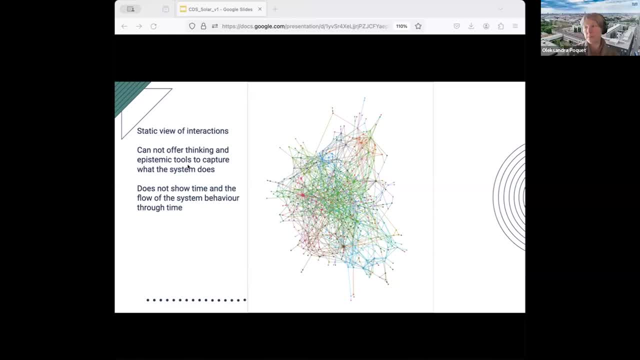 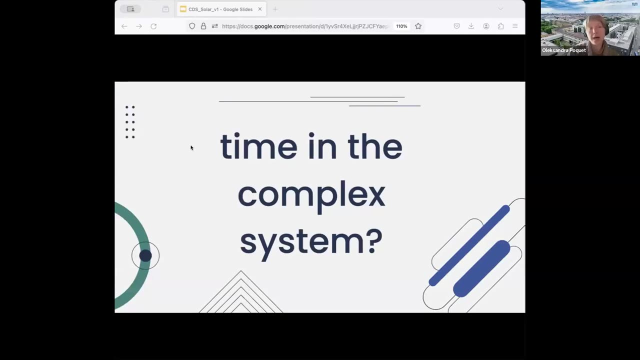 evolution and development, while the image itself only shows a static view of the system. The image, like the one I showed you, is limited in showing what the system does, And so, to understand what the system does, we need to integrate time into this picture. Complex systems are assumed to have. 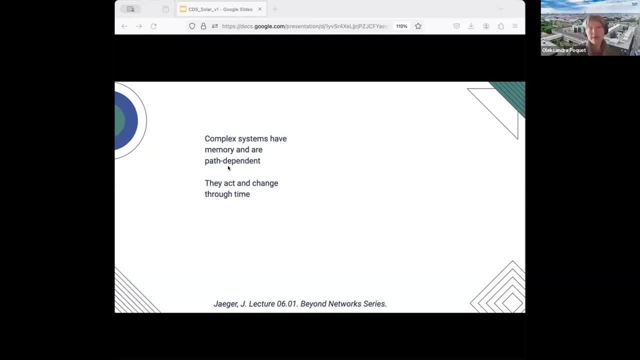 memory and to be path dependent. And that means that the history of behavior of a system affects its future. And that means that the history of behavior of a system affects its future. And that means that the history of behavior of a system affects its future, And it also is assumed. 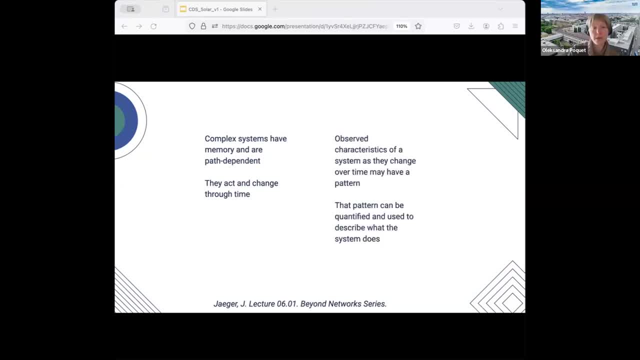 that these systems act and change through time. Characteristics of these changes may have a stable pattern, and this pattern can be used to describe what the system does. And so, with this thinking about time and how to bring it into the definition I suggest to use for the modeling purposes. 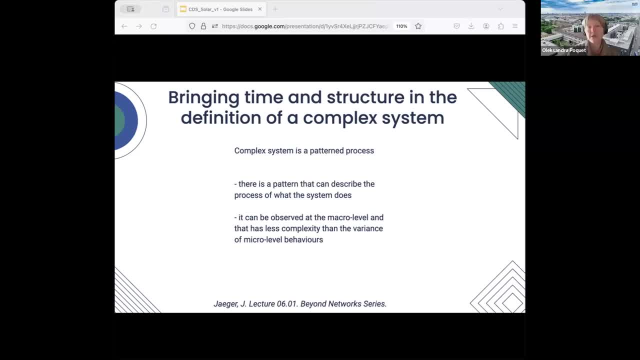 the definition by Johannes Jäger, who argues that for modeling a system, a complex system can be defined as a patterned process. And if we define a system as a pattern process rather than a thing, then we presume that there is a pattern of what this system does and that this pattern can be observed at a macro level. 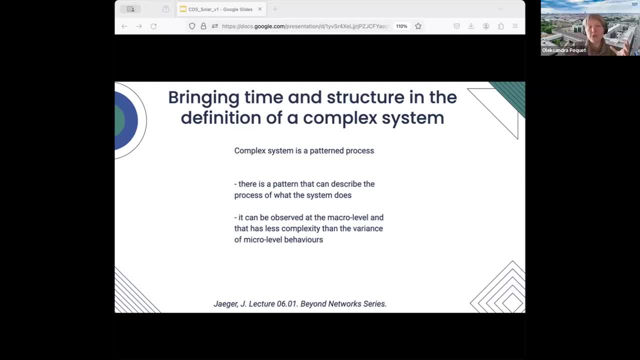 where we need fewer or where we need less information to describe that pattern of behavior and that this pattern can be observed at a micro level. but there we need a lot more information. There's a lot more complexity As to what's happening, but importantly, it means that we then define a system as to what it does. 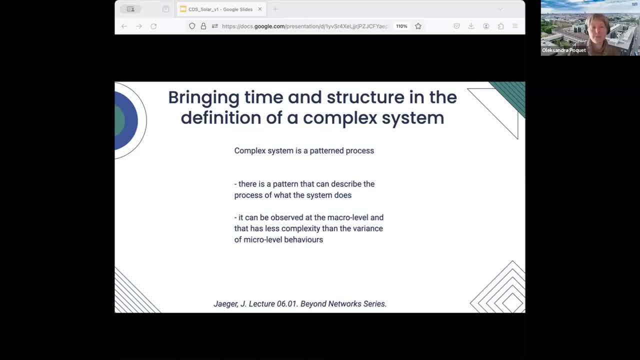 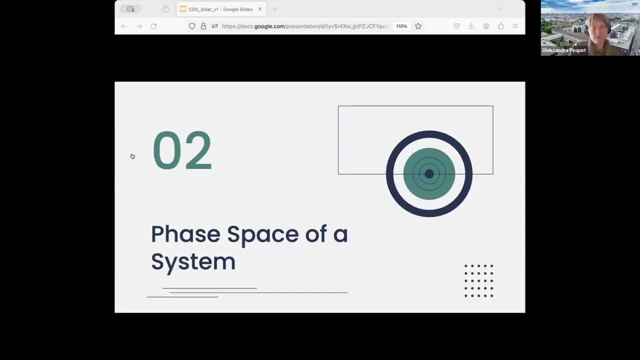 rather than what it is, again for modeling purposes. And so to explain how to model what a system does through time, I will introduce this idea of a phase space of a system. Again, this is just one idea from the complex system repair to our, and we chose this one in order. 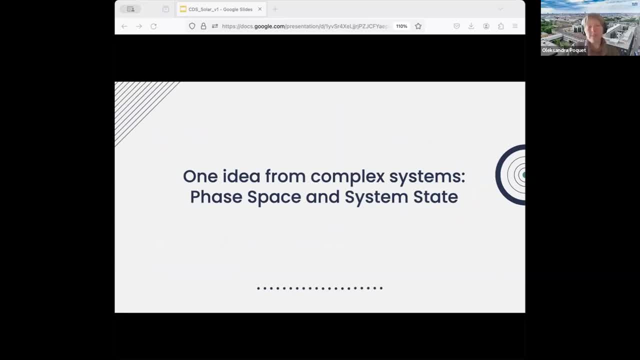 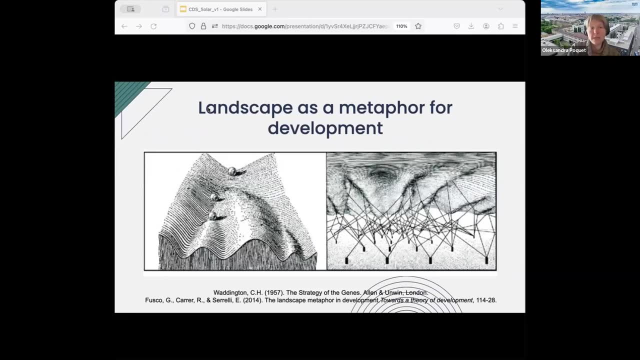 to explain the theoretical assumptions behind the examples that will be presented later in the talk. So, So, first let's talk about the landscape as the metaphor for development and a systems trajectory through it. Developmental trajectory refers to the trajectory of the past that the 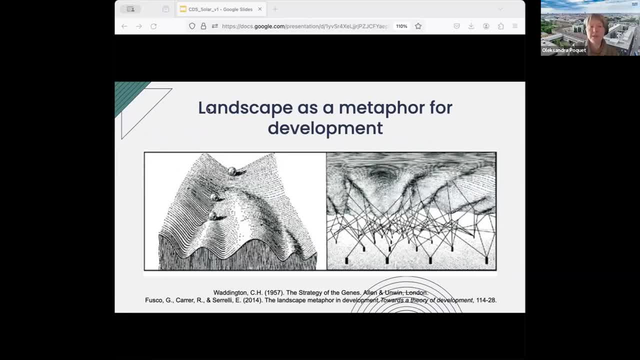 system takes to move through the space of all possible behaviors it can have. So I use the seminal metaphor from epigenetics here on the slide. The landscape, such as on the left, is the metaphor for all possible places where the ball can roll on, and the ball represents a system. The shape of the landscape is contrary. 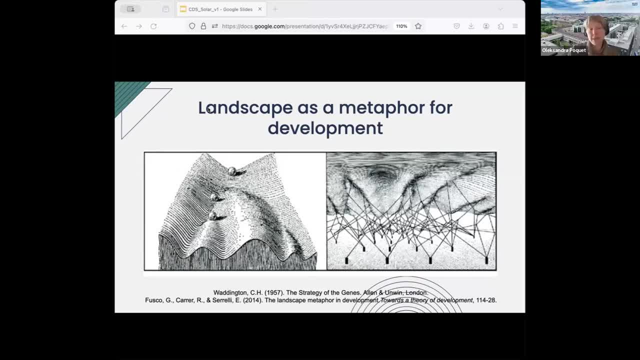 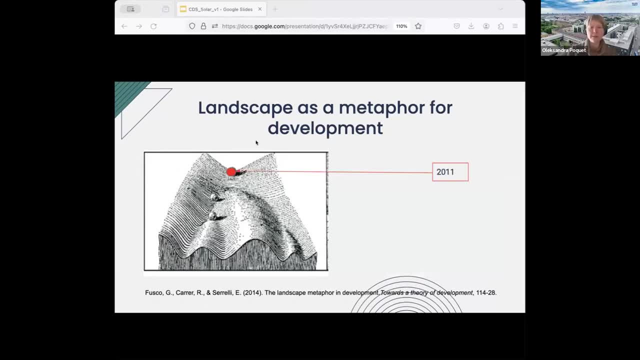 and constrained by forces or specific perturbations, as illustrated by the image on the right of the underbelly of the landscape. Now going back to my example about the public knowledge of learning analytics, if we capture the position of the system of public knowledge creation in 2011,, then 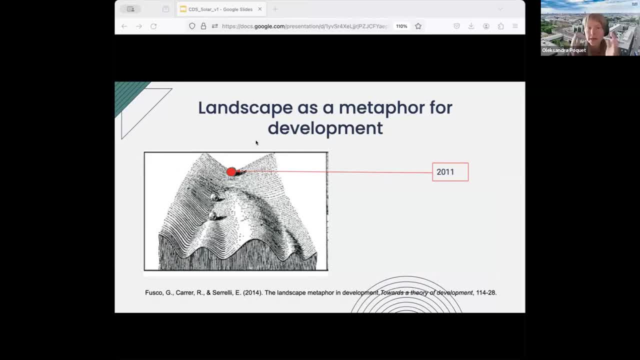 we can just put the red ball where the system is, that entire system of knowledge in 2011.. And we can continue adding information about where that system is in other years. So yellow ball represents the same system in 2013.. Blue ball represents the same system in 2014.. And so you see the trajectory of knowledge. 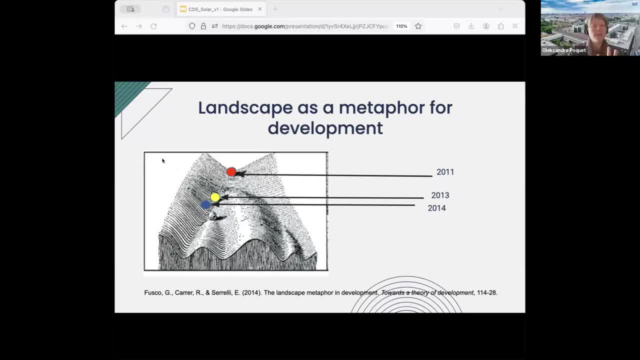 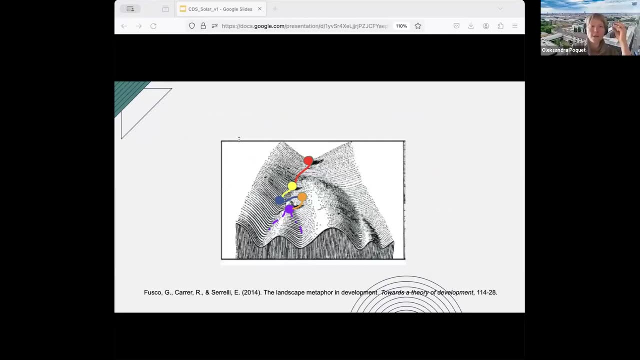 production process captured on the landscape. This is still a metaphor. We're not talking modeling If we continue adding time points when our system is captured, so in different years we can over time look at how this trajectory unfolds on the landscape of all possibilities. 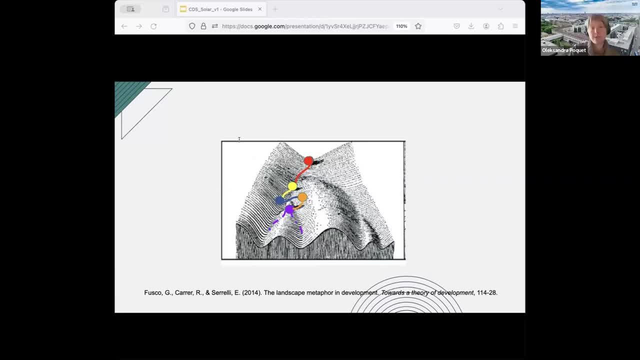 So the past of how the ball, this specific system, has evolved is called the developmental trajectory, And here time means color. Well, color means time, And the position of a system on this landscape at any given moment represents the state of a system at 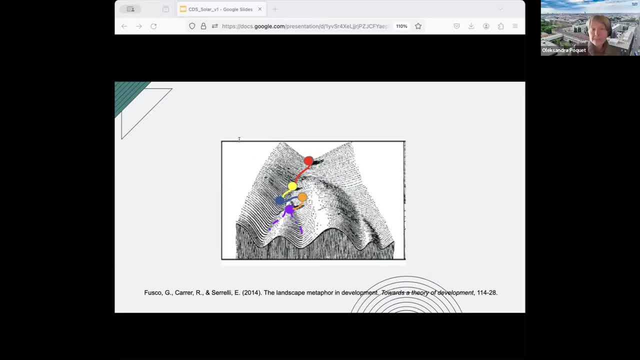 that moment And we can see that right now where it is in purple. it can go because of the shape of this landscape, because of the way these possibilities are constrained by some other forces. It can either go right or left, for instance, or anywhere within those possibilities, But also besides these states. 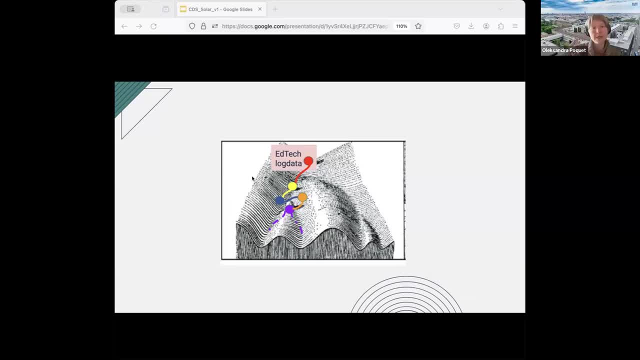 so the momentary measures on the landscape. we can talk about phases, And phases describe the state of the system qualitatively and they differ from each other. So, for instance, in 2011,. maybe, knowledge creation, where the red ball was best described, by building on educational technology. 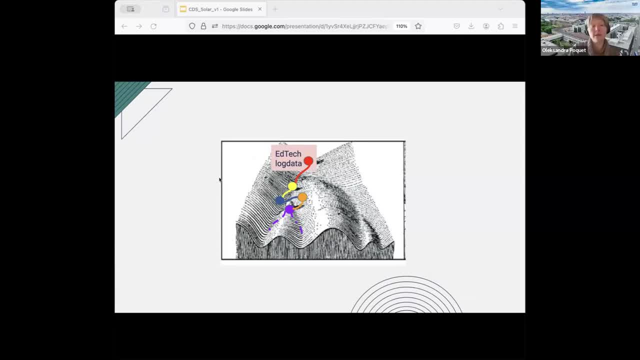 literature and types of data that come exclusively from digital learning, so log data, for instance, right, But maybe if we want to describe qualitatively where the ball of the system of knowledge is in 2019, it can be described in completely different qualitative. 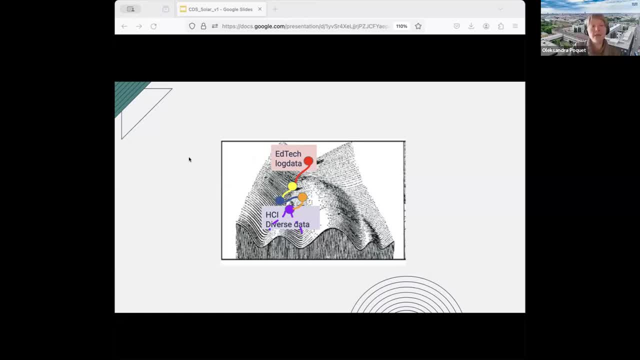 terms such as inspired by HCI literature and participatory design, or characterized by the diversity of data used And maybe although the state of the system. so the momentary measures for yellow, blue and orange balls are kind of different quantitatively but they share. 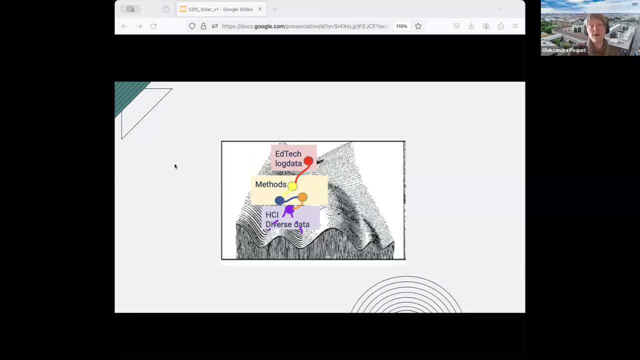 the same qualitative properties. So the domination, for instance, of methodological questions over questions about theory of learning, or maybe the use of log data, with just a few examples of multimodal data. So this is just a pure example to try and illustrate a few simple ideas. well, 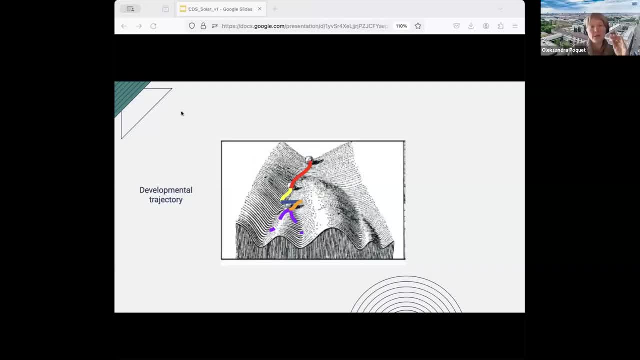 not so simple, but a few useful ideas. let's call it that way. First is this developmental trajectory that is the state of a system at a given time, And third is the phases that describe multiple related states of the system, And I hope that the images went through correctly, because it sort of 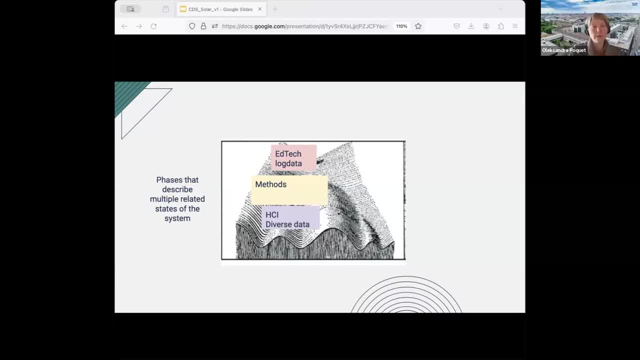 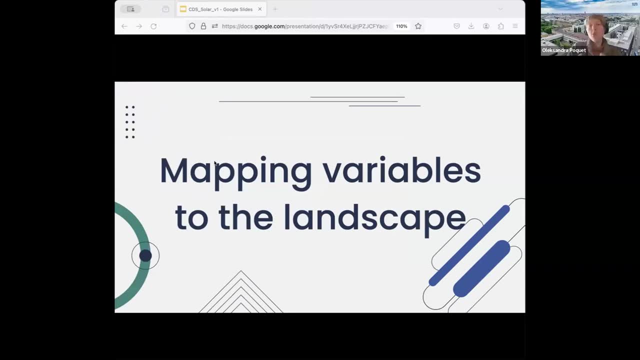 summarizes the notion of what I'm trying to say, And then the question is: okay, well, this is a nice metaphor, Sasha, thank you very much. But how do we move from there to modeling this, What this system does? or, put it another way, how do we move from the metaphor to modeling this? 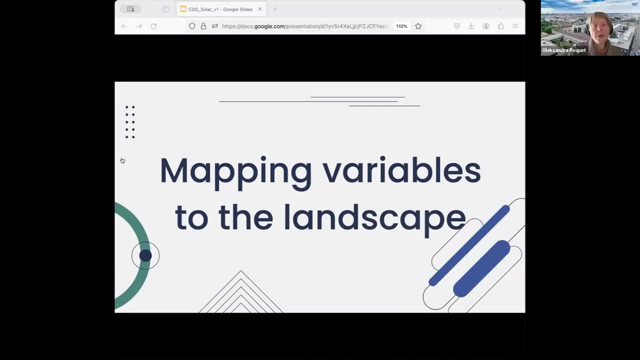 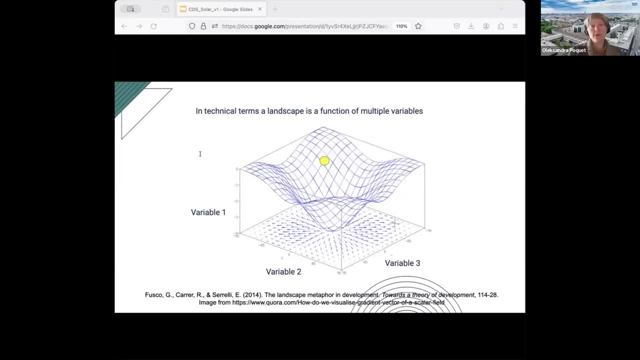 Thanks, Sasha Sure. So modeling is, let's say, another form of a statistical process or a conceptual process, the development of a process of learning and then, of course, the development of a knowledge creation. So we do this through multiple variables, But we can also do this through: 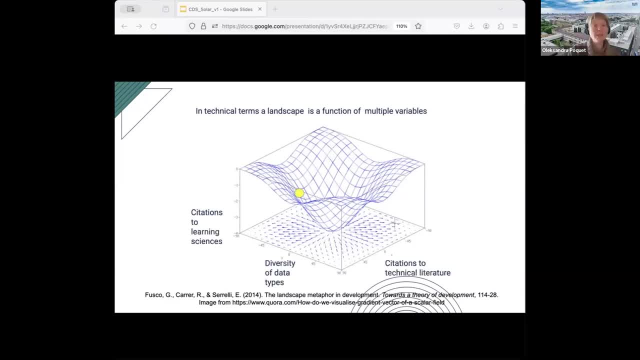 multiple variables, And then we can talk about it in more detail at a different time points. So let's say, for example, you want to use a method to know the state of the system at its given point in time, all right. So if you can imagine that you have what we call a process in 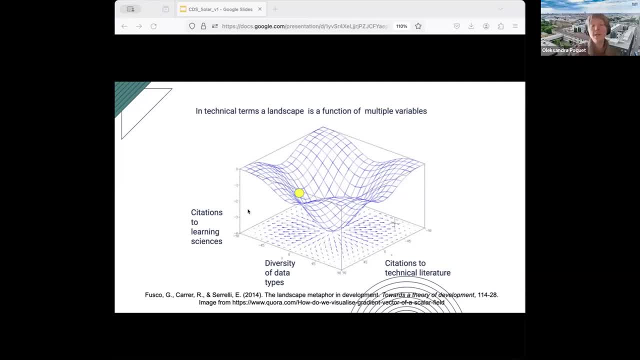 this way, the process of the system, for example. So with that, create a work, create a model, create a to learn in science, literature in that tier, diversity of data types reported in that tier and number of citations to computer science. 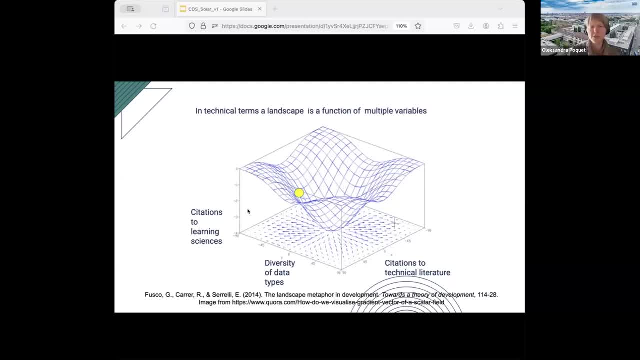 and statistics in that tier, You should already be thinking: well, how did she pick these variables? Well, yes, it is a little bit arbitrary in my case, but if you are really modeling something in relation to learning that it's a non-trivial process of variable selection. 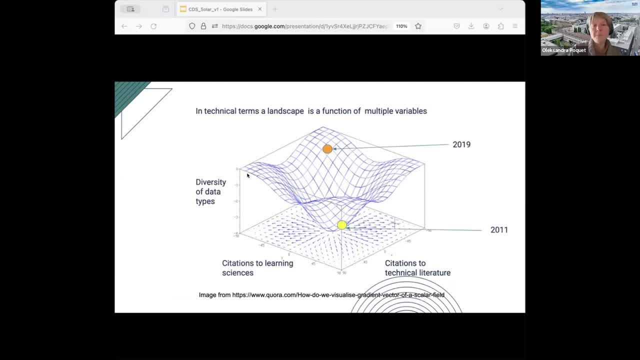 in relation to an analytical purpose or a given theory. But here we continue my metaphor. So I have these three variables in a space and I measure these three variables at a point in time in 2011 and 2019, which allows me to position where my system 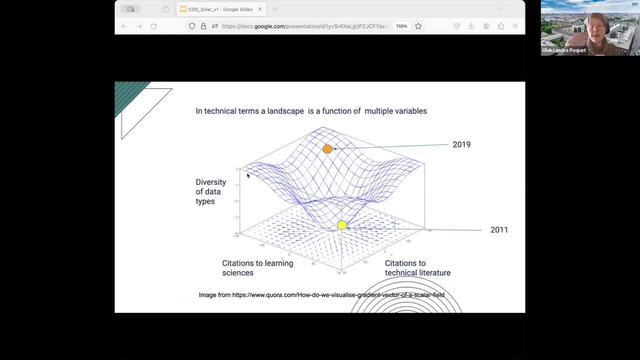 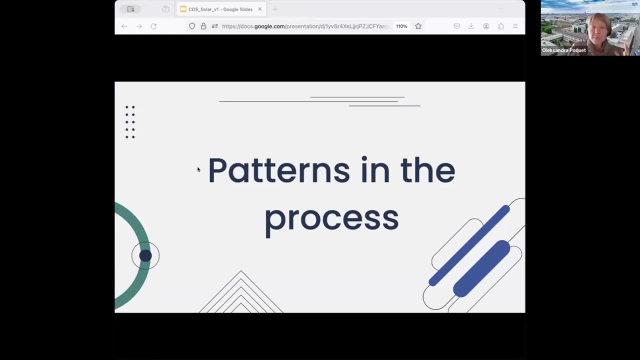 the state of knowledge or knowledge creation is located in relation to all possibilities. And now if I want to understand complex system as this pattern process of what the system does on this map, then I can ask questions: well, what are the regularities? 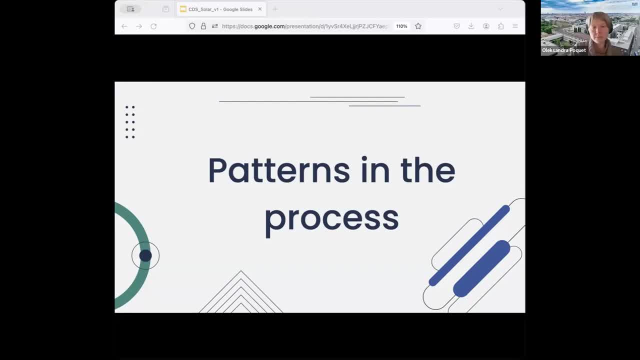 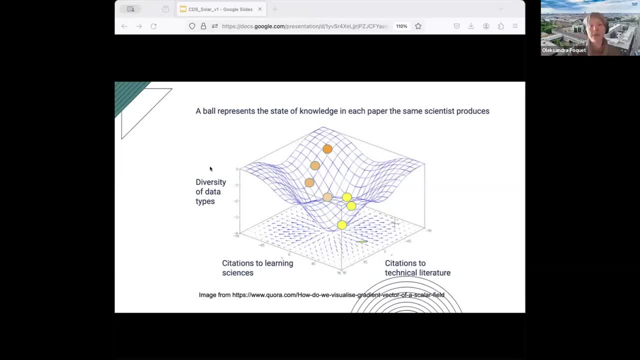 and how my system moves through this landscape, And so, to demonstrate this idea, I'm changing the example slightly. So, instead of considering all learning analytics papers, let's just consider my paper. So some my knowledge production process. So these are the papers. 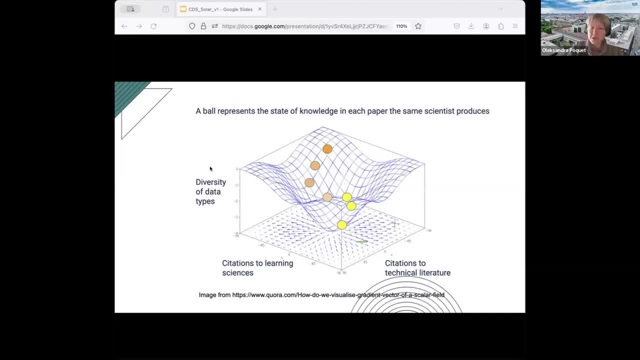 each paper is can be characterized by this learning science citation, computer science citations and diversity of data used- And I'm mapping my papers over time on this landscape And you can see that my first paper may be yellow- is defined by particular characteristics. 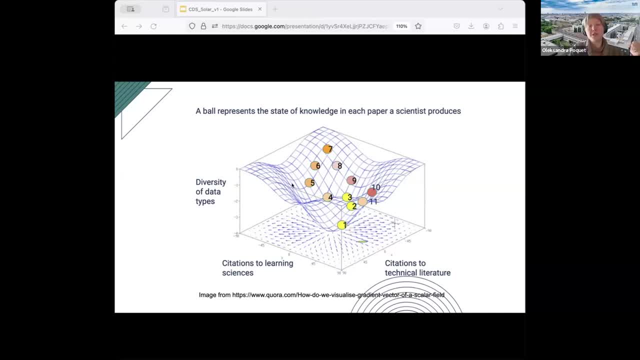 Second is still yellow and third is the same, but fourth paper starts changing. Seventh paper is in a completely different place And then maybe my paper still oscillate back to the type of papers I was writing as I was in the beginning. Of course, all of this can be represented as time series. 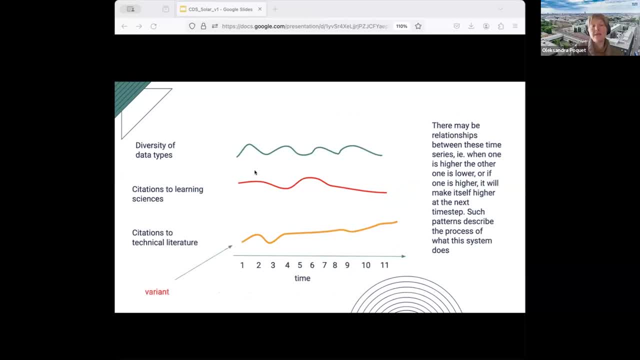 rather than mapped on the three-dimensional space, And in this case we will see a lot of variance from momentary measures at a time series level, at a micro level, And we will see a lot less sort of variance at the level of quality. 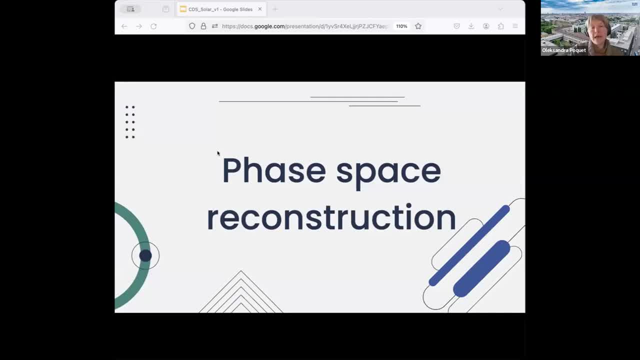 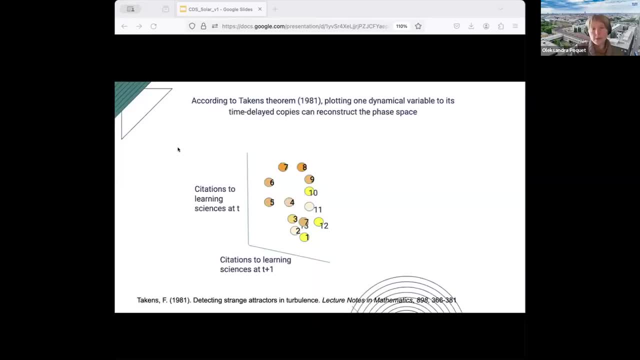 but we will see a lot more variance at the level of the quantitative descriptions, And that brings us forward to analysis of these patterns in the phase space and system states. So there is one important assumption that exists when we talk about phase space of a complex system. 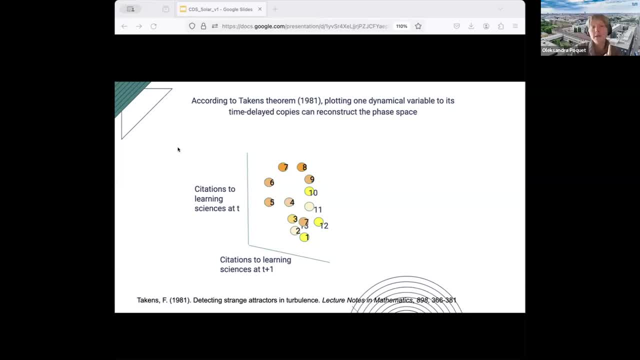 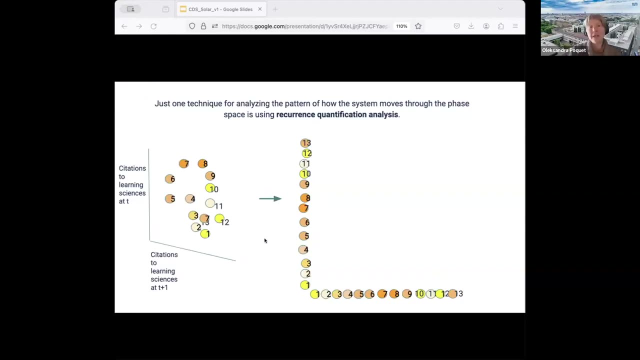 and that is the dynamics of the system, can be reconstructed only by using time-delayed copies of a single time series, of a single observable dynamical variable of this system. Meaning I only need one time series mapped to itself and I only need one time series mapped to my space. 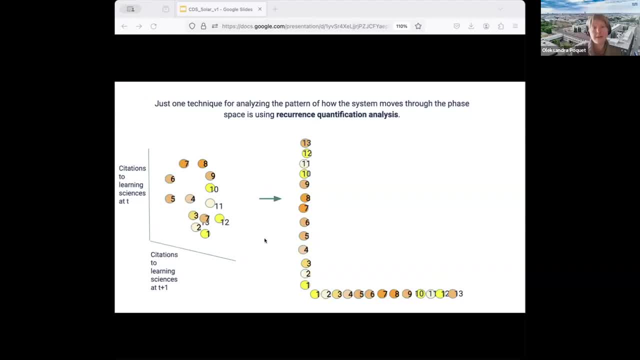 And so one technique for analyzing this process is recurrence quantification analysis. So here on the left, you see that my space is no longer defined by different variables, but it's the same variable, the same time series and its copy, with a time lag. 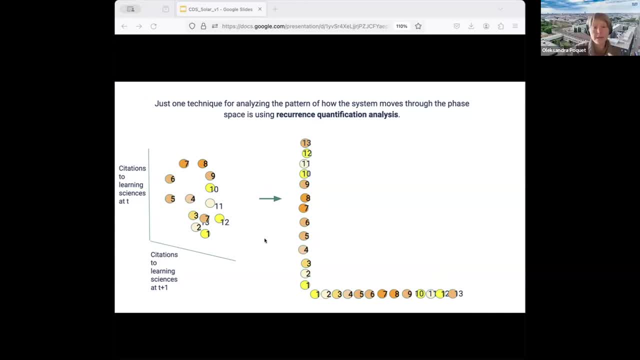 or with a time at a previous point, for instance at the next point, And I can add more of these copies, which our QA allows us to do, and quantify how the time series repeats themselves, And on the right I have an example that tries to illustrate that. 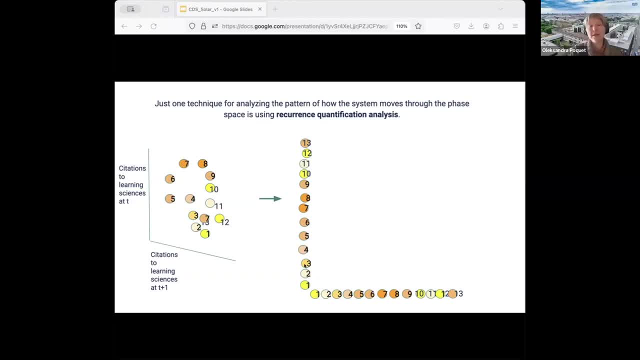 So I put these time series horizontal and vertically and every time the number repeats, like you can see here in an image. So for instance, when my paper one is yellow as a particular measures of citations and diversity of data use, then at point my paper 10 is similar. 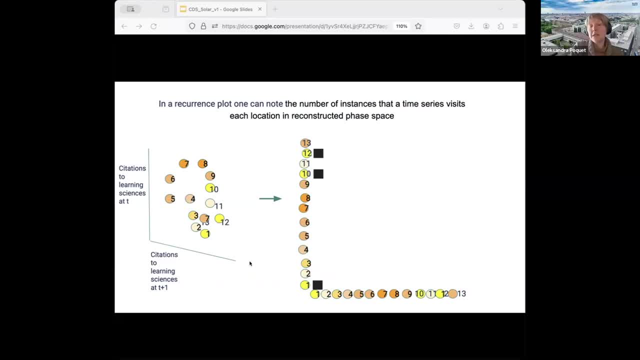 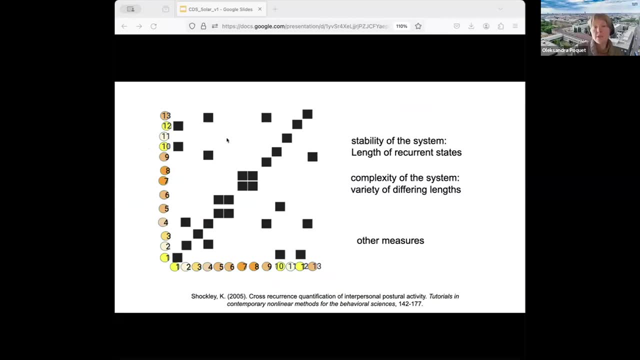 So I put a dot there. my paper 12 is similar. If I continue doing this with every paper and mapping it to itself, I could have a visual that quantifies the number of times the system revisits the same states within the facial space. 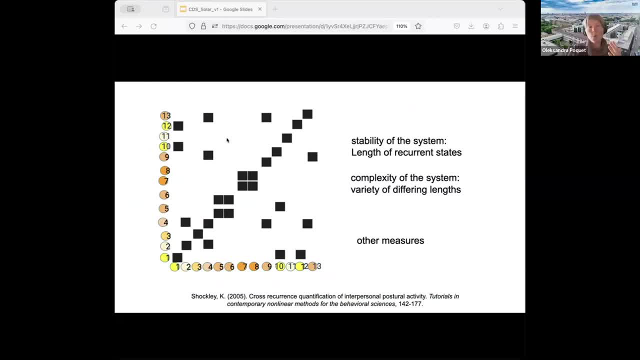 So these are patterns of recurrence, can be quantified and they are known in to describe something about how the system moves through the face spaces. It's stable, is it predictable, is it deterministic, is it perturbed, et cetera, et cetera. 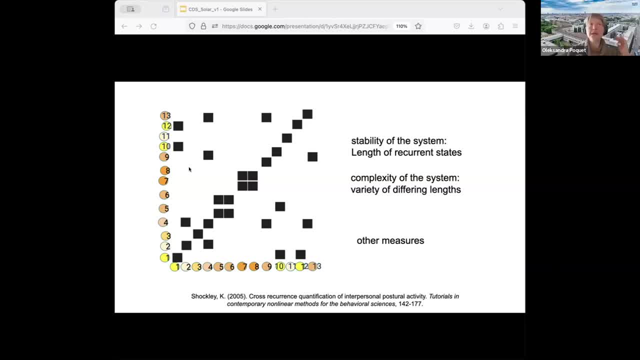 And so now I hope this introduction is sufficient, that at some level you get a grasp of some of these ideas and then you can see how they can be translated into some specific applications of learning, analytics, research. So I pass the words to my colleague, Liz here. 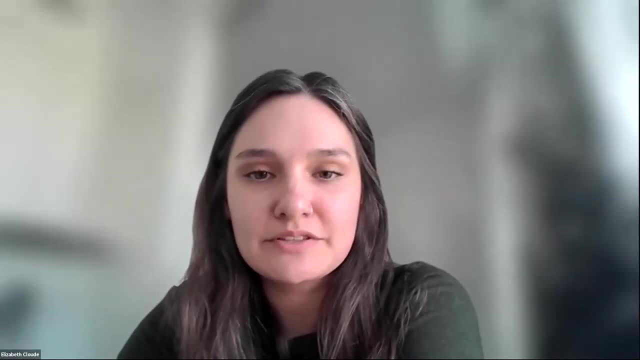 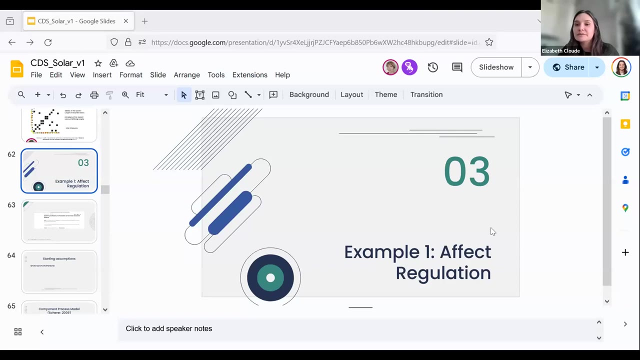 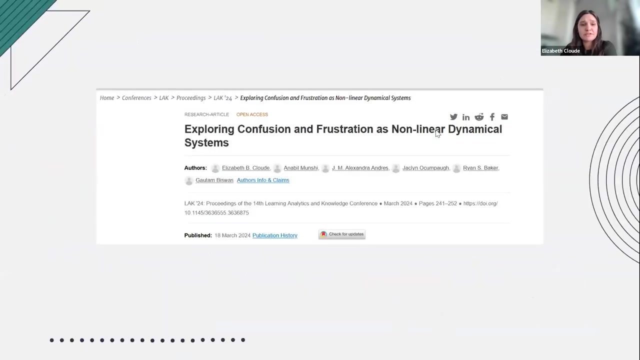 Okay, hi everyone. Please give me a brief moment to share my screen. Okay, you should be seeing a slide deck now. All right, so let me begin by first introducing you to a publication I'll be talking about. It was just published a few weeks ago. 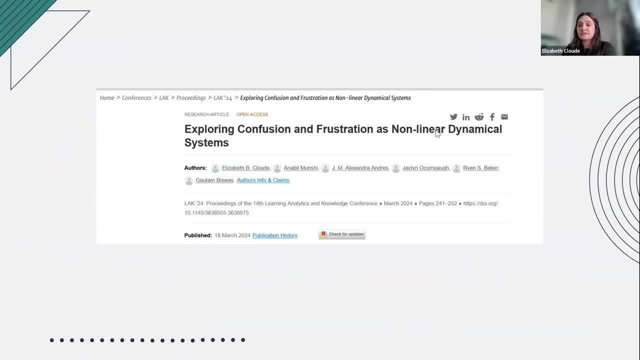 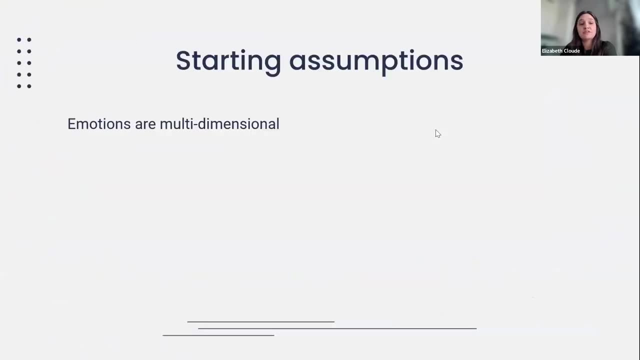 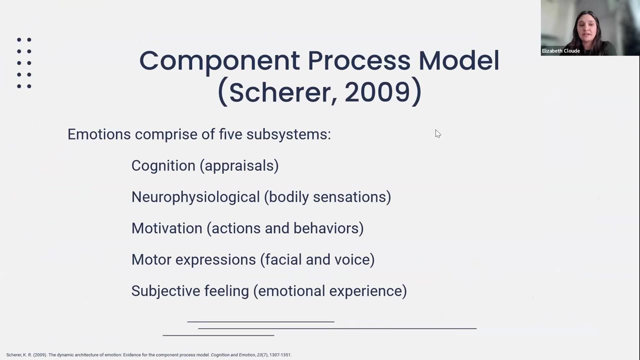 at the LEC Conference called Exploring Confusion and Frustration as Nonlinear, Dynamical Systems, And so this paper has. one leading assumption is that emotions are multidimensional in nature, And this was guided by the component process model developed by Scherer in 2009.. 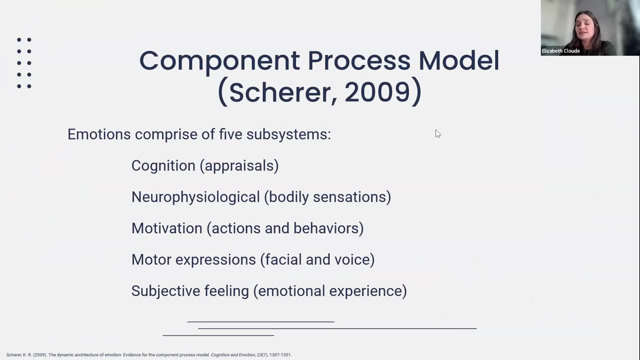 It ultimately states that emotions are multidimensional in nature, So emotion comprises of five subsystems and these subsystems are described by cognitive. So thinking about the cognitive appraisals that learners may be making regarding stimuli in their environment. Also, the neurophysiological facet of an emotion. 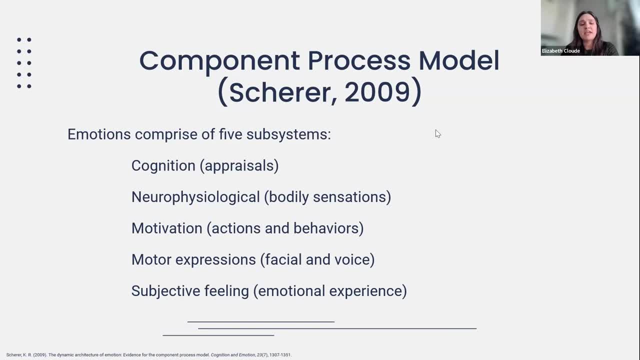 So, thinking of the central nervous system, motivation components, the behaviors that might underlie an affective state, as well as the motor expressions and the subjective feeling, And that all of these subcomponents, these subsystems of the emotion, are deeply interconnected. 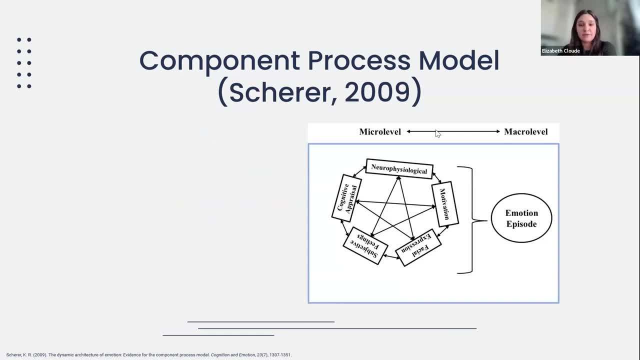 Meaning that they are interacting constantly over time at a more macro level And that, based on this interaction, there may be synchronized changes between either all or multiple components And that, based on this synchronization, it gives rise to a more macro level state, which we would come to know as an emotion. 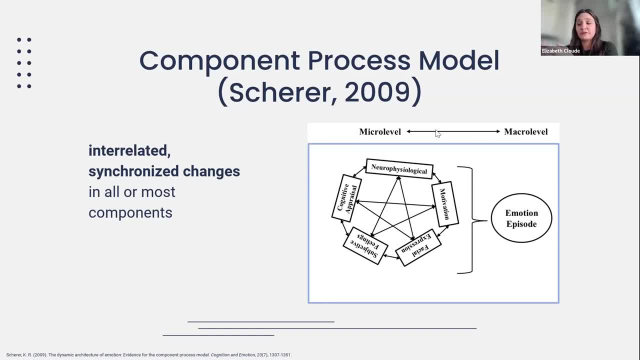 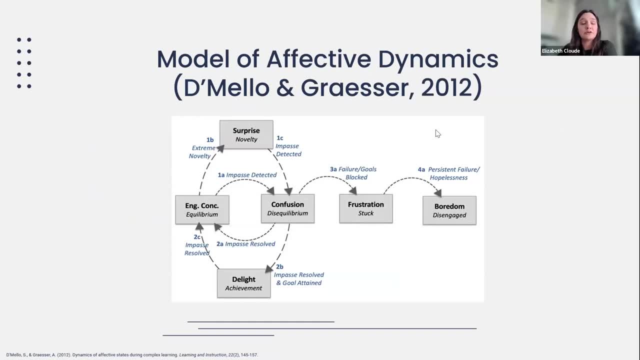 And so thinking about emotions within the context of learning, particularly within the context of digital learning environments. one of the most popular frameworks that's used to study emotions some of us may be familiar with is called the model affective dynamics, And this model is based on the notion. 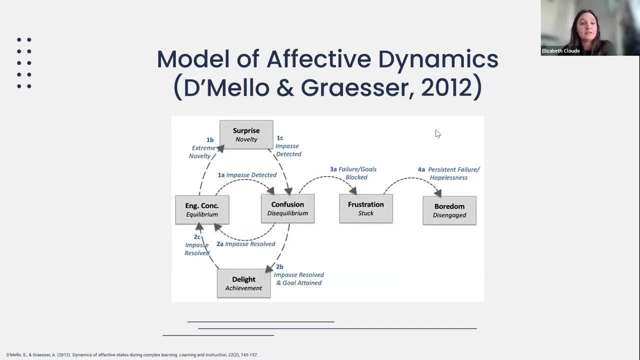 of cognitive disequilibrium. that's coined by Jean Piaget, And so it ultimately states that a learner encounters a state when they encounter a state of uncertainty when they're trying to assimilate new knowledge into their existing schema, then they would engage into a state of cognitive disequilibrium. 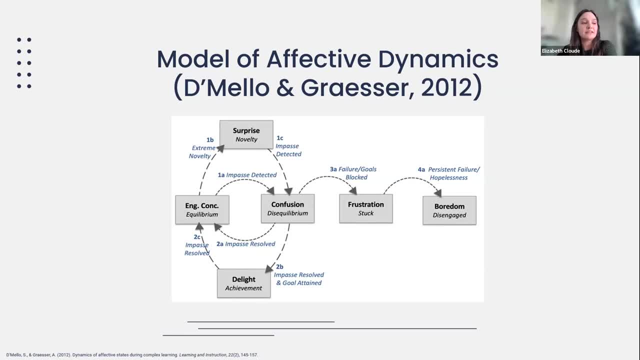 And the extent to which they can resolve that cognitive disequilibrium or regulate it back to a state of equilibrium would determine the extent to which that affective state is beneficial or detrimental to the learning process. So you can see here a student is engaged with the material. 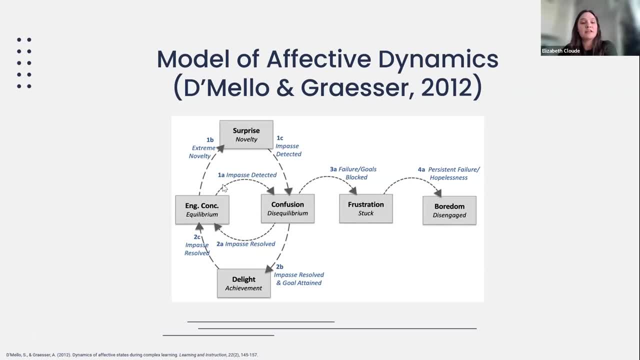 they're entering. they're in a state of cognitive equilibrium. When they encounter that impasse or state of uncertainty, they would transition to a state of disequilibrium. When they can transition or resolve that disequilibrium, they would transition back to a state of equilibrium. 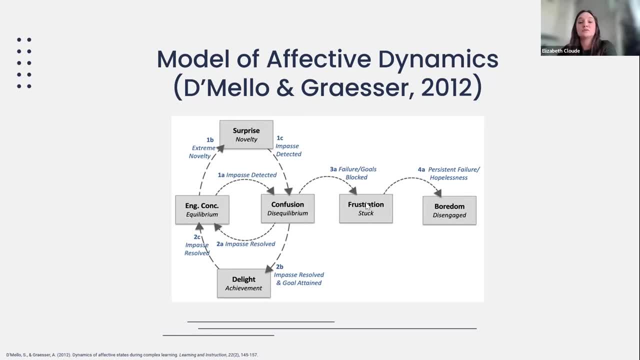 But if they're unable to resolve that state of disequilibrium, then they would transition into a state of frustration and boredom. And so, based on these particular affective sequences, a lot of research and research researchers have tested this empirically And across the board. 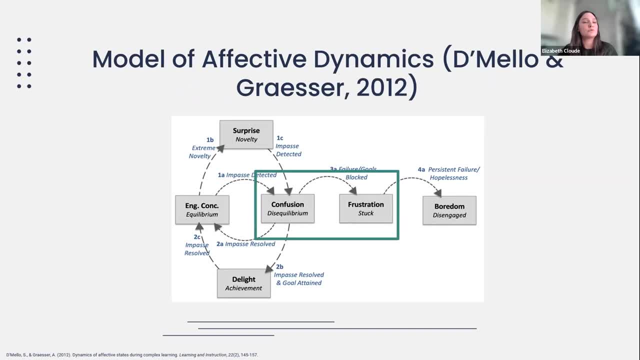 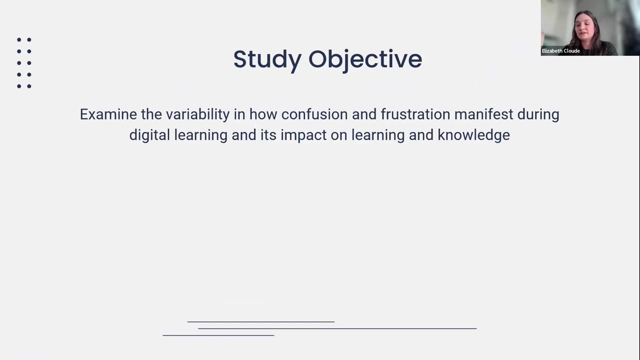 a lot of research find there's inconsistent results, particularly around transitions between confusion and frustration, So that sometimes these emotion categories are beneficial to learning, but other times they're detrimental, And so in this particular paper, we wanted to really examine variability that may underlie these different emotional categories. 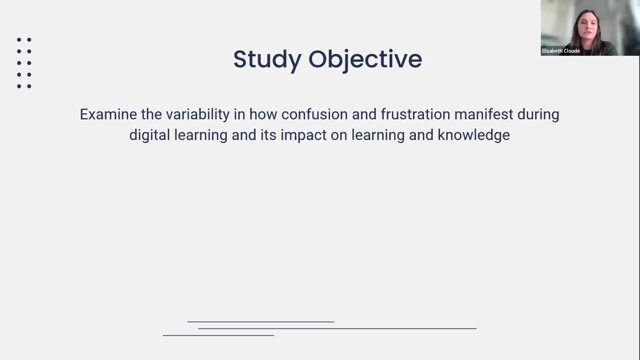 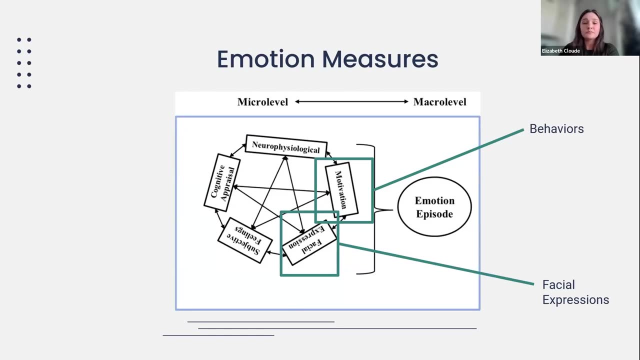 and whether they impact learning and knowledge differently, particularly with the context of digital learning. So for our specific study, we examined, referring back to that component process model, two components of an emotion. We looked at the motivation component by defining confused and frustrated behaviors. 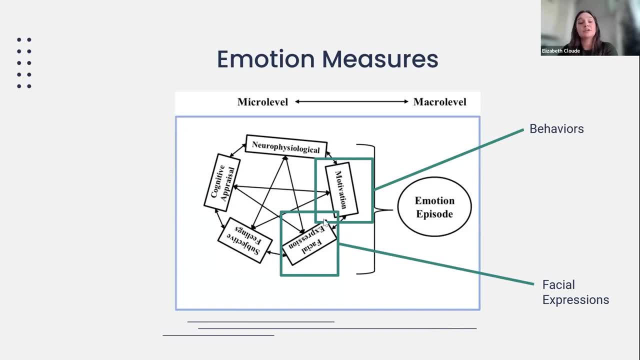 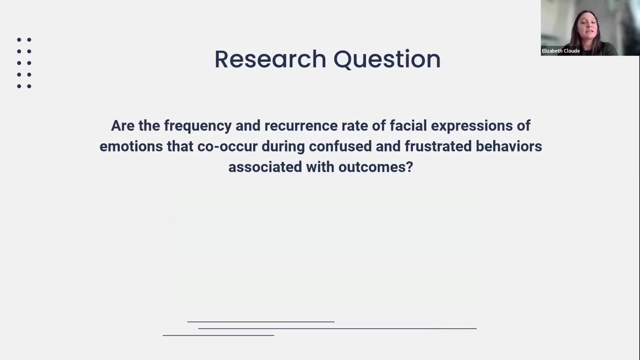 and how they co-occurred with frustrated- excuse me- facial expressions. So again tapping into that motor expression, And so our leading research question for this paper was: are the frequency and the recurrence rate of facial expressions that co-occurred? 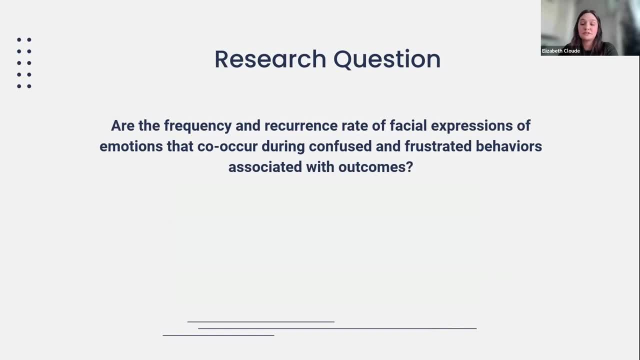 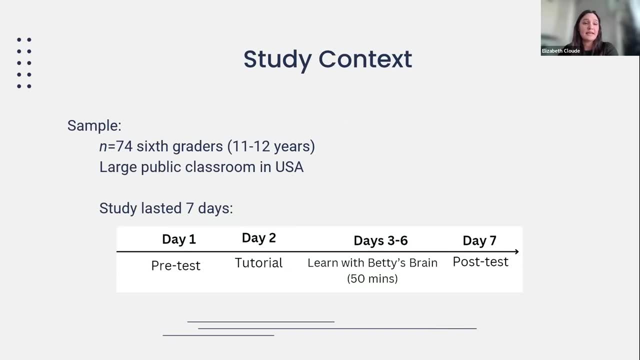 during those confused and frustrated behaviors, is it associated with outcome measures, Outcome measures being learning and knowledge, And so, in this study, we captured a sample of 74 sixth graders at a large public classroom in the United States, And the study lasted approximately seven days. 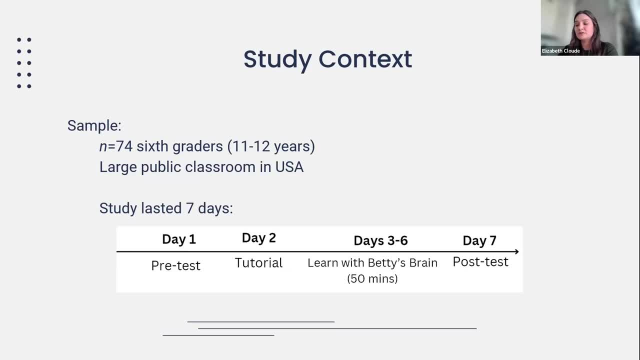 So on the first day, students completed a pretest assessment of their knowledge. This was specific for climate change, which was the topic of study. Then, on the next day, they completed a tutorial So they would learn how to utilize the tools in the interactive digital learning environment. 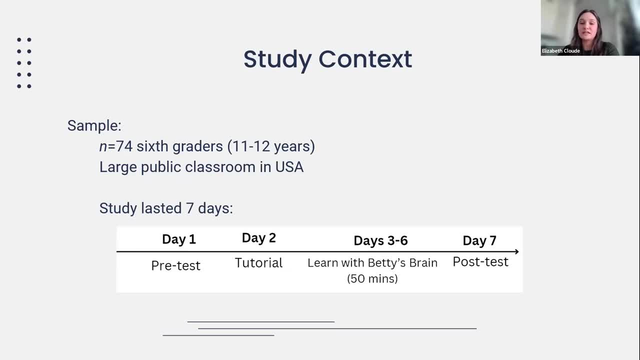 called Betty's Brain. I'll touch on Betty's Brain just briefly on the next slide. And then they learned with Betty how to use Betty's Brain for approximately 50 minutes each day over the course of three days, And on the last day they completed a post-test assessment. 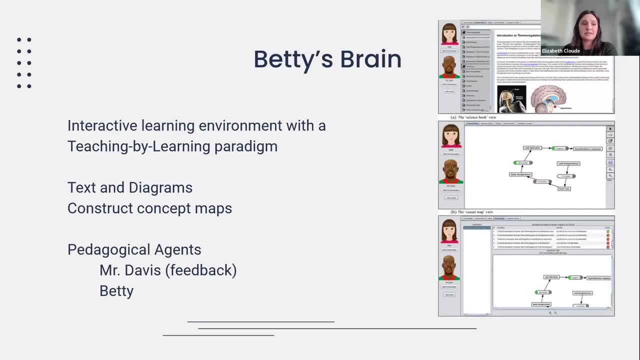 And so, in terms of Betty's Brain, I wanna touch on its interactive nature, which follows a teaching by learning paradigm. So students essentially enter this environment. They're asked to learn about climate change by engaging with texts and diagrams. Then, from engagement, 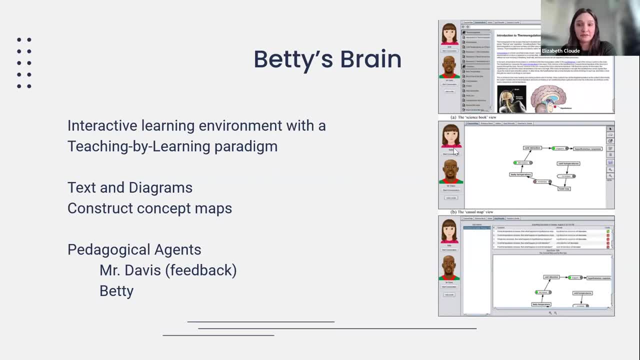 they're asked to teach the concept maps, to teach Betty, the pedagogical agent on the top hand left side of the screen, about climate change by essentially replicating their mental model, And then they can assess the accuracy of that concept map by referring to Mr Davis. 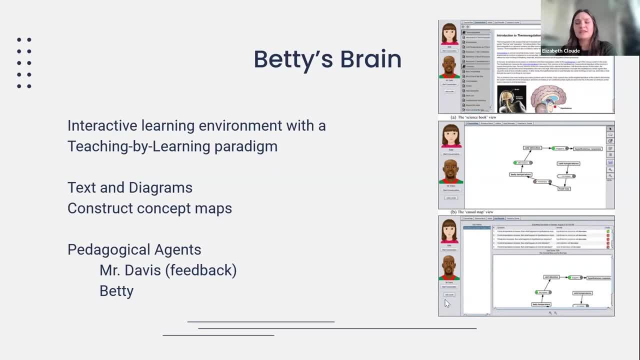 who provides information on which components may be accurate. And then they can take that information, that feedback, and revise those concept maps by either referring to the material again or simply providing new notes to connect to their concept map. And so, based on the highly interactive nature, 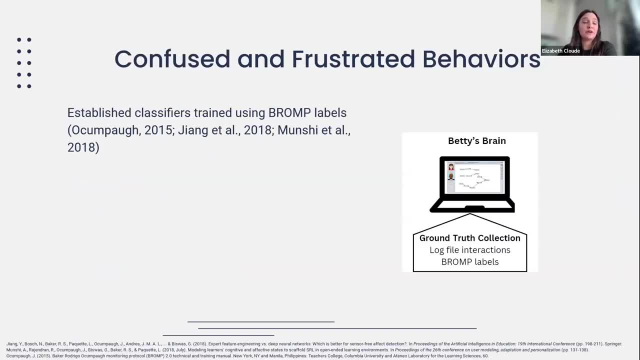 of this environment. this is the information we use to classify whether or not they were confused or frustrated. So what we did is, in a prior study, we used established classifiers that were trained using Brompt labels. So again in an earlier study, 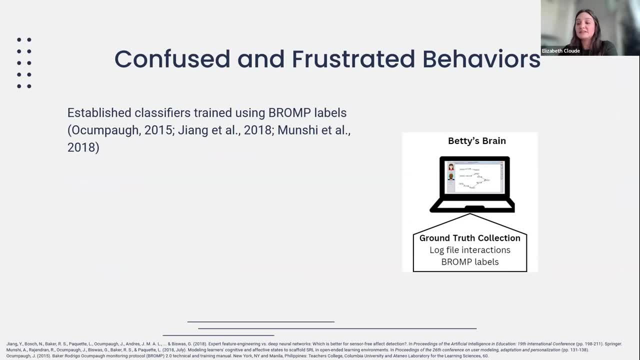 researchers went into the classroom as students were learning with Betty's Brain, and they essentially created labels of the amount of time or the frequency at which students were confused or frustrated. What am I trying to say Now? Brompt is actually a field observation protocol. 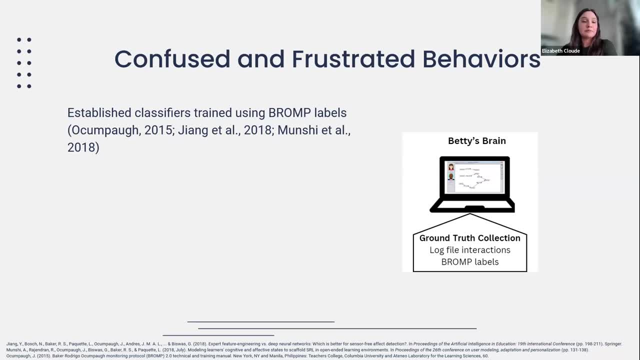 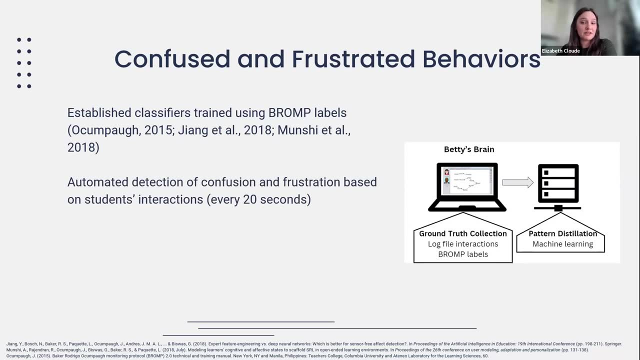 So students are able to use it, So researchers can actually go directly into the classroom label these affective states. And so what we did is we took those labels, we mapped them on to students' interactions with Betty's Brain And then, in this particular study, 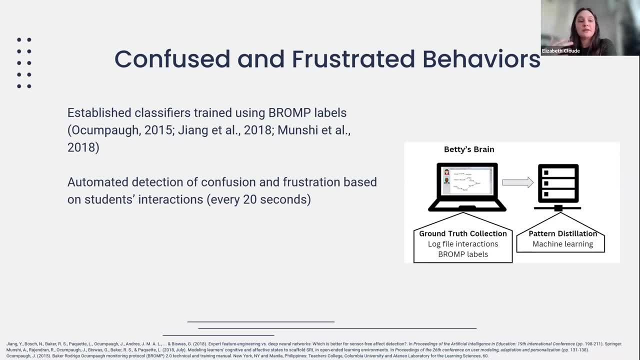 we created automated detectors of confusion and frustration, So this is solely using students' interaction data. So approximately every 20 seconds we had a confidence rating of the likelihood that confusion was present or frustration was present. So during these confused and frustrated behaviors, 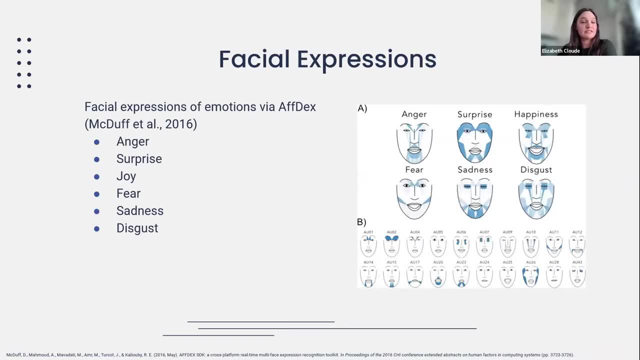 we captured students' reactions. We captured students' facial expressions using AFDEC's automated facial recognition software. The software was designed using Paul Ekman's facial action coding system. So what we did is we captured those six emotions- facial expressions- based on a configuration. 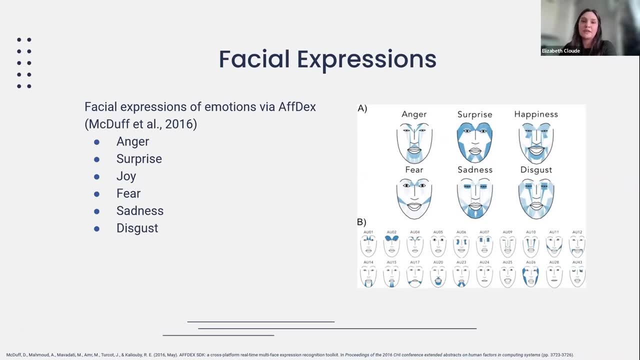 of their muscular contractions over the course of the learning session. And so, in order to examine the co-occurrence of those facial expressions, as they co-occur with those frustrated or confused behaviors, we used a method that Sasha briefly talked about. 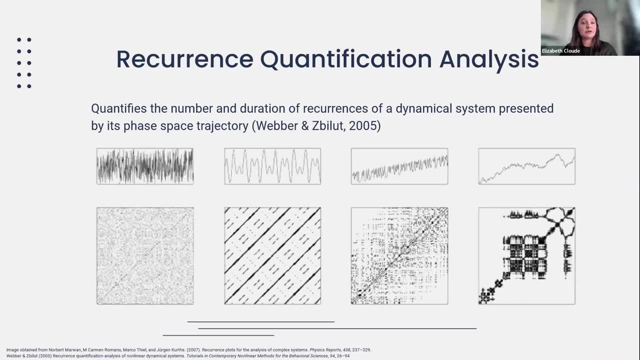 recurrence quantification analysis And again this quantifies the number and the duration of recurrences that occurs within that phase space trajectory. So you can see, here I wanted to provide a brief example of the sort of variability we can get in examining the temporal structure of a time series. 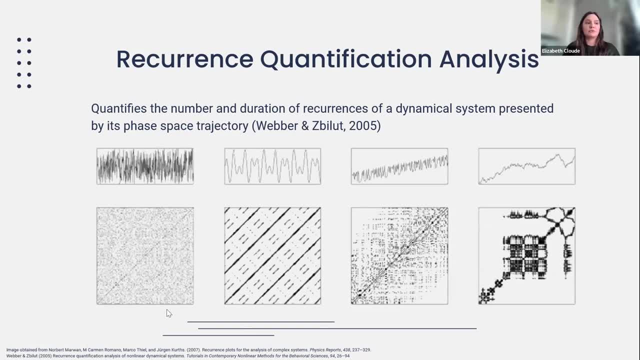 So for example, in this first plot here we can see the noise is quite random, So there isn't a lot of recurrence. However, in the next plot you can see the recurrence is quite periodic. In the third plot we have sort of an autocorrelation. 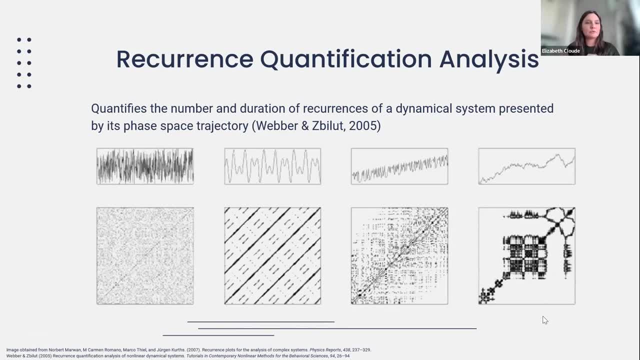 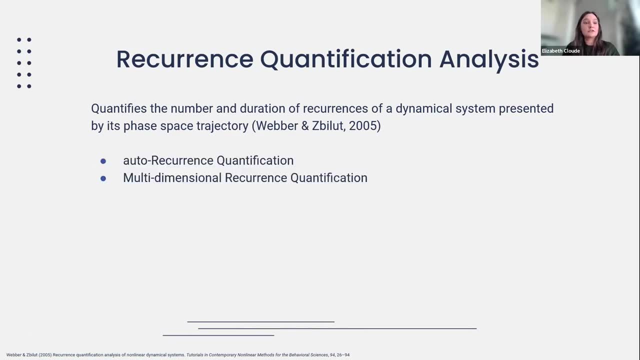 And then on the final plot, we have more of a chaotic recurrence. So we wanted to use this method to really look at the variability in that co-occurrence between our two emotion components. So what we did is we used auto-recurrence quantification. 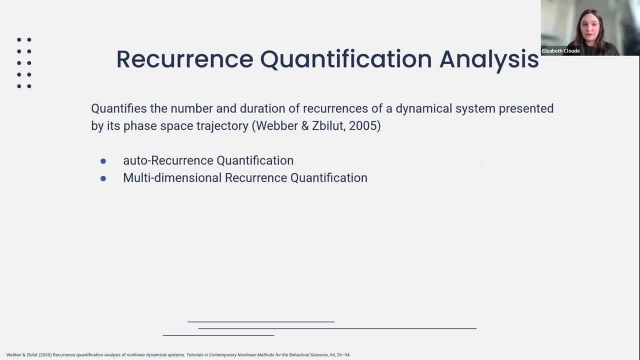 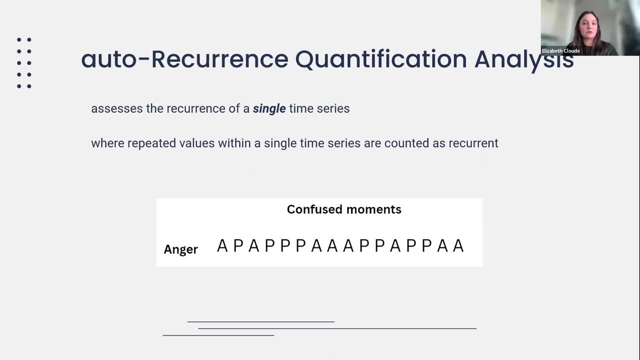 and multidimensional recurrence quantification. I want to unpack those just a little bit. Auto-recurrence quantification deals with assessing the recurrence of a single time series. So in our particular example, during those frustrated moments, we captured their anger. They're facial expressions. 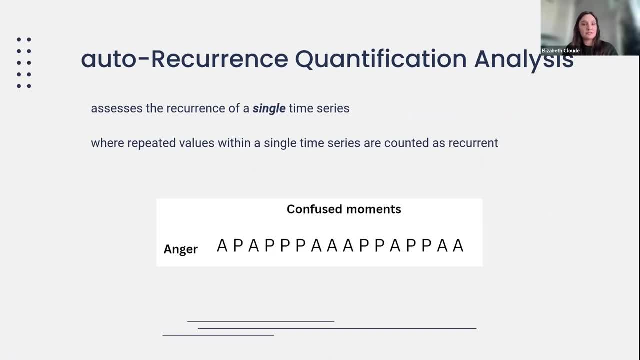 And so A and P here are used to denote the absence or presence of the facial expression. So in this analysis we can capture patterns at which that presence of facial expression were recurring over time during confusion, And then similarly for multidimensional recurrence. 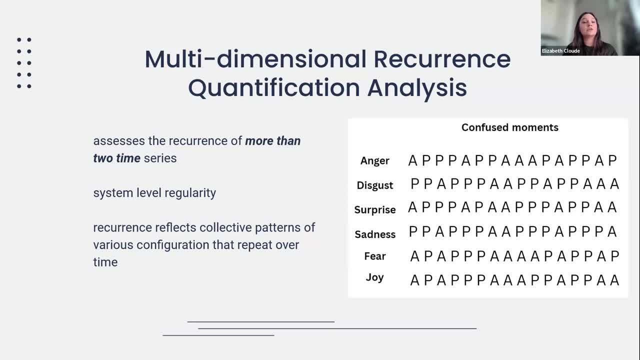 this method allows us to assess more than two time series so that we can capture sort of system-level regularity across all of those facial expressions of emotions, as you can see during those confused behaviors. So we can capture sort of the recurrence rate of more collective patterns across all the motor. 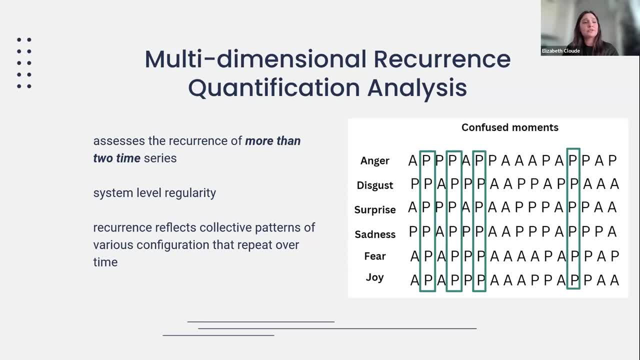 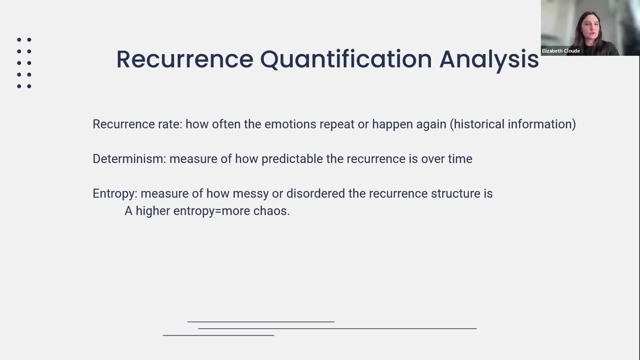 expressions that a student may be expressing, And so through this methodology we can capture recurrence rate metrics. So how often is that emotion repeating, such that we get the historical information of how often it's recurring in that particular state? We also have determinism. 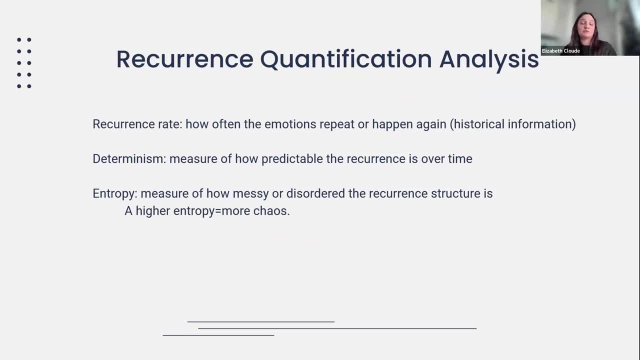 So how predictable is that recurrence over time? And then finally entropy. So this is a measure of how chaotic or organized that recurrence structure is, And so, again, we wanted to look at these metrics in relation to learning outcomes. So we ran Spearman correlations. 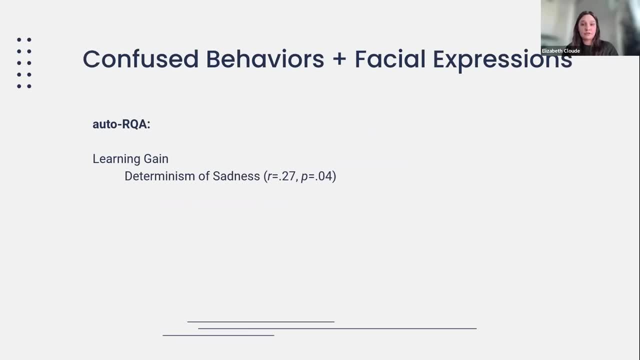 Our first assessment looked at confusion, frustration and the co-occurrence of facial expressions For our auto-RQA. so again looking at that single time series, we found a significant positive relationship between the determinism of sadness co-occurring with confusion. 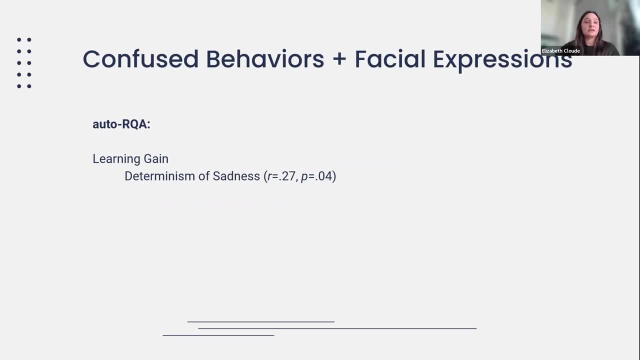 So what that means is that recurrence rate recurringly returning to a state of sadness co-occurring with confusion. it reoccurred predictably, So it was quite regular during the learning session and that this regularity was actually beneficial for learning. 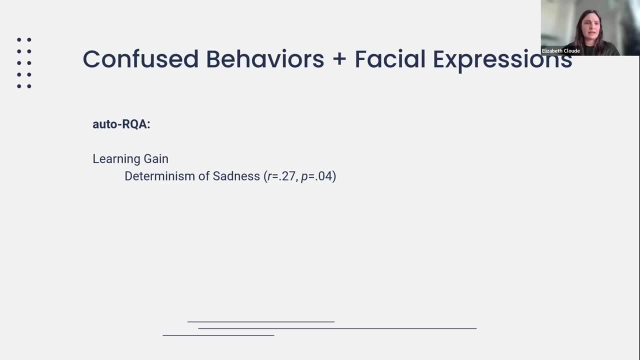 We can interpret this as a student is continuously encountering that state of uncertainty. Again, they're confused, They're in a state of cognitive disequilibrium. If that's happening repeatedly, perhaps they are a bit disappointed in their performance, based on their facial expressions of sadness. 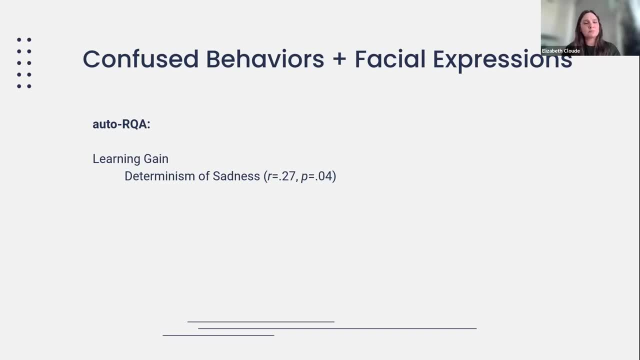 So this is recurring repeatedly. The student may be disappointed, But they could be pushing them to persevere And it could eventually be beneficial for the learning process and learning game. However, when we looked at the multidimensional measures- so those collective measures of regularity- 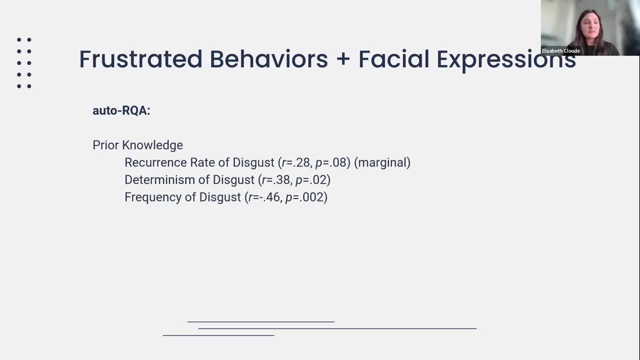 we didn't find any significant relationships with our outcome measures Now transitioning to frustrated behaviors and co-occurrence of facial expressions. for our auto-RQA, we found a significant relationship where students who came in with more prior knowledge to the session was associated with more recurrence rate. 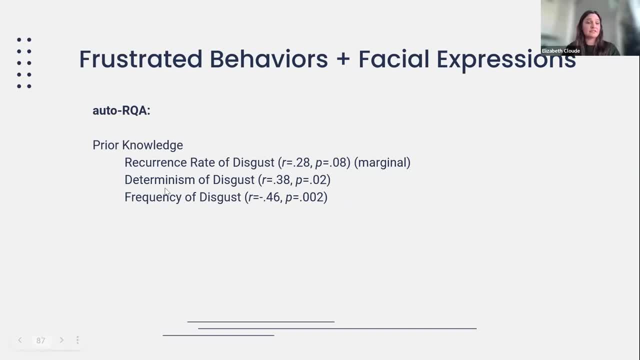 of disgust and more predictive recurrence of disgust denoted by that determinism. So that's what we found. We found that students who came in with more prior knowledge were associated with prior knowledge with the co-occurrence of frustration. So again, the more often that disgust 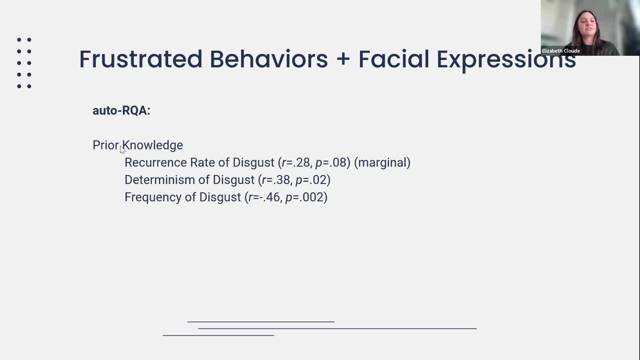 recurred and co-occurred with frustrated behaviors was associated with the student having more prior knowledge. But the less prior knowledge the student had was associated with more frequency of disgust co-occurring with frustration. Now it's important to distinguish frequency from recurrence, because frequency doesn't account. 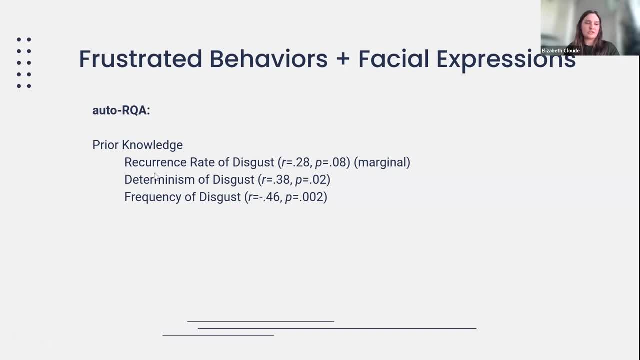 for the historical variation. So a student who has more prior knowledge, they may be experiencing more disgust, co-occurring with frustration, if they had more expectations about performing well during the session But if they weren't performing well, for example, they're recurringly and regularly experiencing. 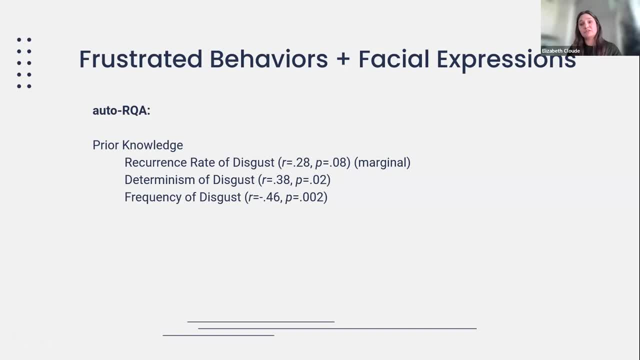 bouts of frustration. they're stuck, they're not able to overcome that cognitive disequilibrium. they may be disappointed in facially expressing that as disgust because they're not meeting up to their expectation because they have a higher prior knowledge. However, if they're not having recurring bouts of that, 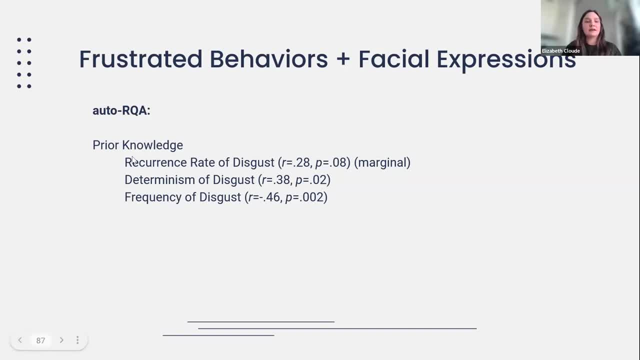 they could just be occurring occasionally, And so it wouldn't be. maybe they didn't have as much prior knowledge or expectations about how they would perform. Now, when we look at its relation to learning gain, we found a significant negative relationship between the determinism, so that recurring 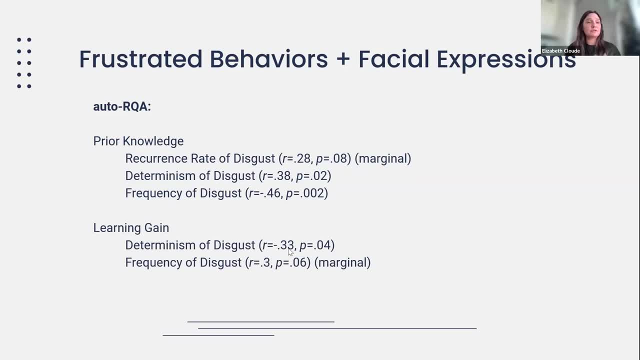 regularly recurring bouts of disgust with frustration was negatively associated with learning gains. In contrast to that, that frequency of disgust co-occurring with frustration was positively related to learning gain. I think this is really important to distinguish and take note of, because the determinism would indicate. 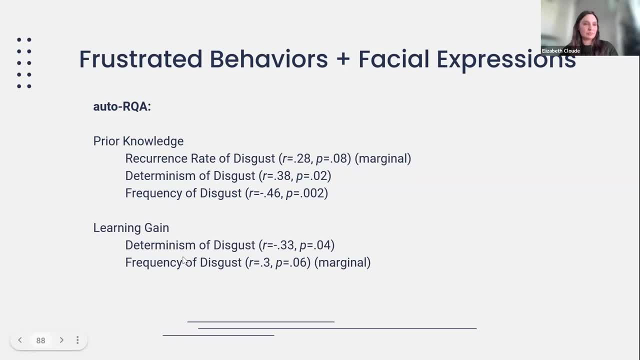 there's a recurring bout of disgust, with frustration, that could indicate a regulatory problem. if it's continuously and regularly recurring And again that regulatory problem might indicate they're not able to regulate that cognitive impasse and they might be stuck, which would be detrimental to their learning process. 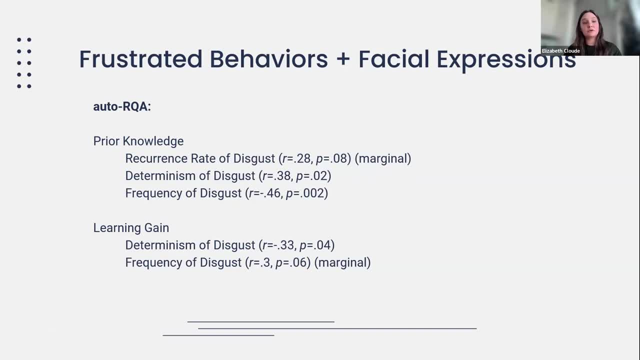 In contrast to that, if it's just a frequency of disgust co-occurring with frustration, there wouldn't be a historical pattern of recurrence there. So again, that might not be a regulatory problem and was actually beneficial for their learning, gain of the information. 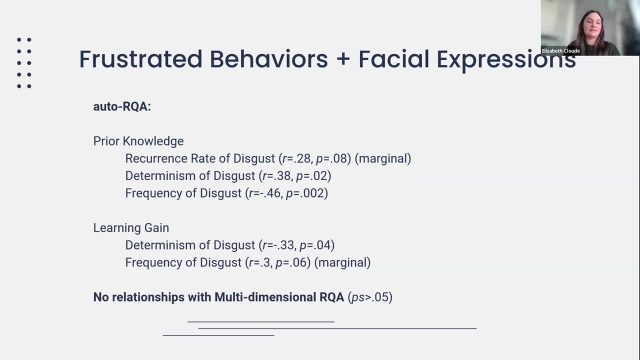 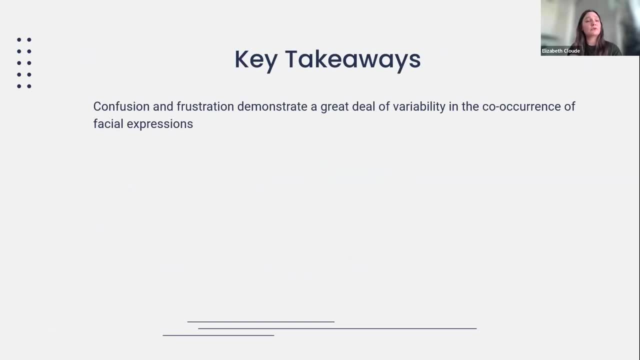 So what can we take away from this? Sorry, we also didn't have relationships with that collective measure here, But an important key takeaway from this is that confusion and frustration demonstrate a great deal of variability with how they co-occurred with facial expressions. 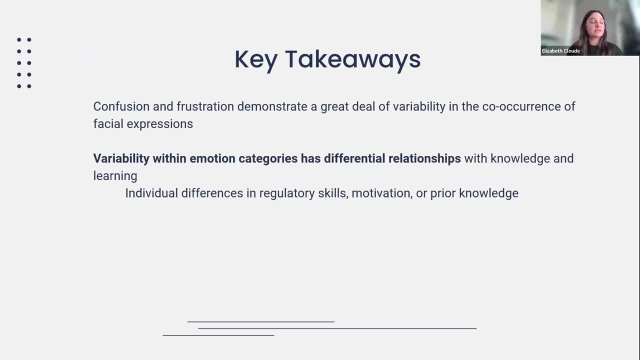 And that this variability within these emotion categories had a different relationship with knowledge and learning outcomes, And that this could be due to differences in emotion regulation skills, differences in motivation or even prior knowledge, as we saw, And that recurrence quantification could provide really valuable insight. 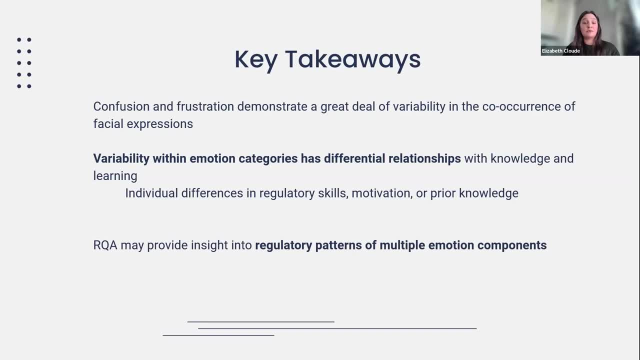 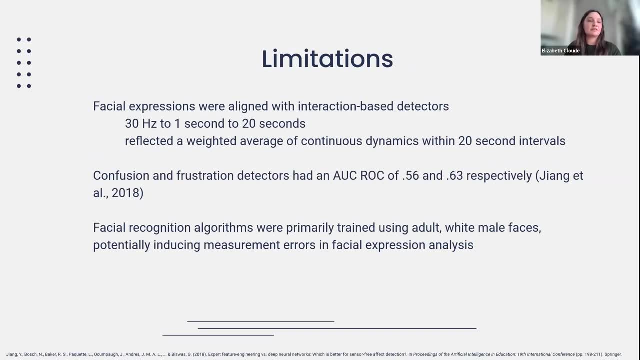 into discovering those regulatory patterns that may occur within one or multiple emotion components. However, this study is not without limitations. We should keep this in consideration. is that our facial expressions were aligned with those interaction-based detectors Which captured frustrated and confused behaviors every 20 seconds. 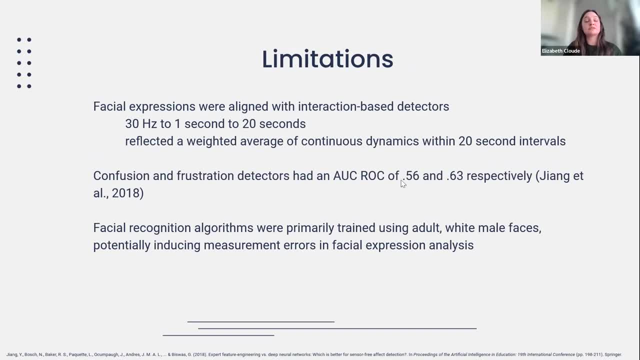 So we actually took a weighted average of continuous dynamics of those facial expressions to align them with our 20-second interval measure of behavior. So we could be missing some dynamics within that weighted average. Also, our detectors had an AUC-ROC of 0.56, 0.63.. 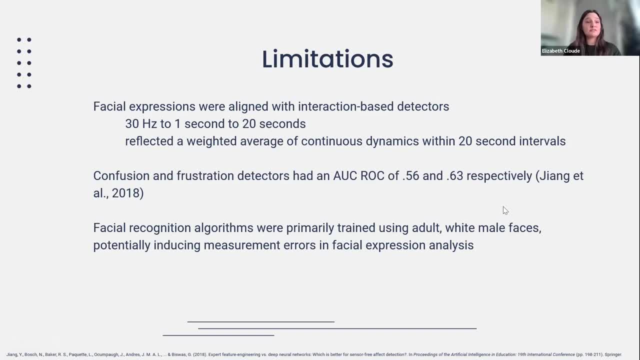 So we could have missed some confused, frustrated behaviors, But it did perform above chance. And again, facial recognition algorithms may present some measurement errors because they're solely trained on adult male faces. And again, we captured sixth graders in the study. 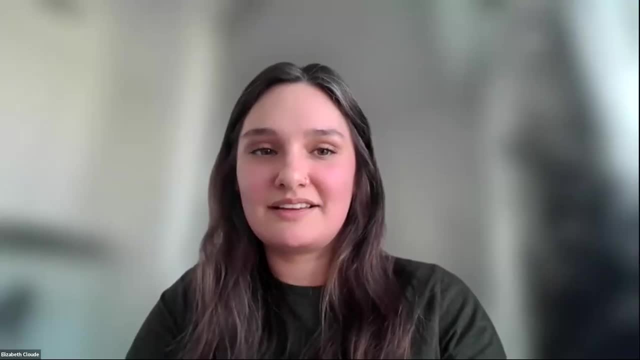 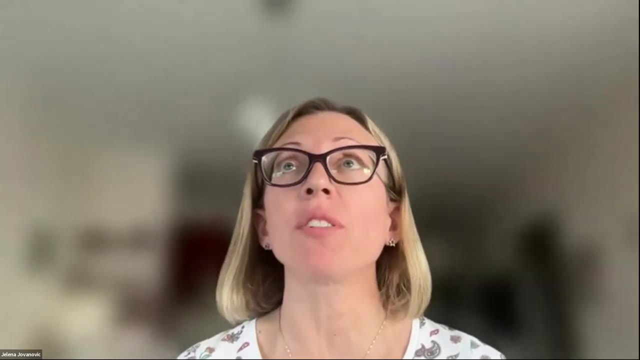 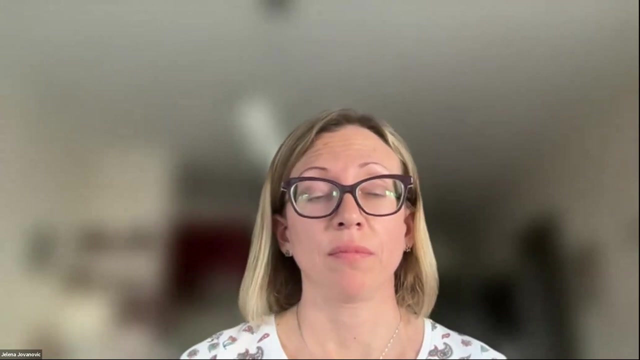 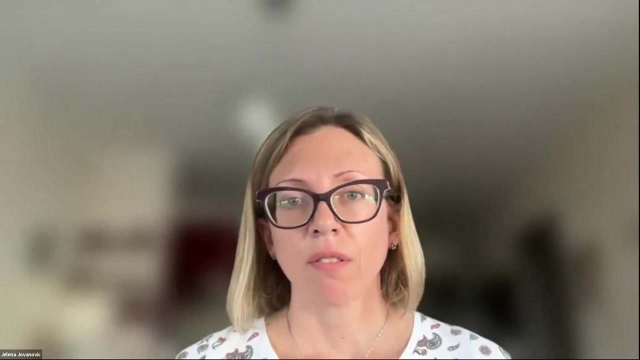 That concludes my example. I will pass the puck to Jelena. OK, thanks. So, hello everyone. Just give me a second to start the slides And, of course, to share them with you. I've got the slides And I'll give you a second to start the slides. 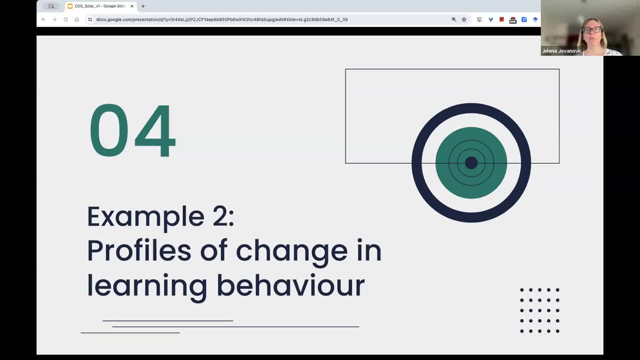 But I'll let you do that first. So please go ahead and start the slides. OK, I hope you see the slides now. OK, I will now present the second example, which is about profiles of change in learning behavior And, as Sasha mentioned at the beginning, 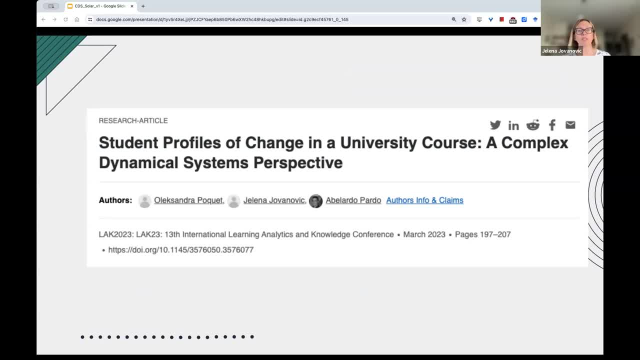 this example is actually based on the paper that Sasha Bellardo and I had at last year's LAC, so LAC 23.. And the title of the paper is Students' Profile of Change University Course: Complex Dynamical Systems Perspective. 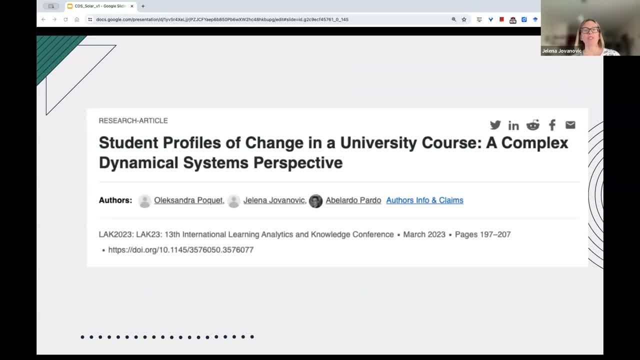 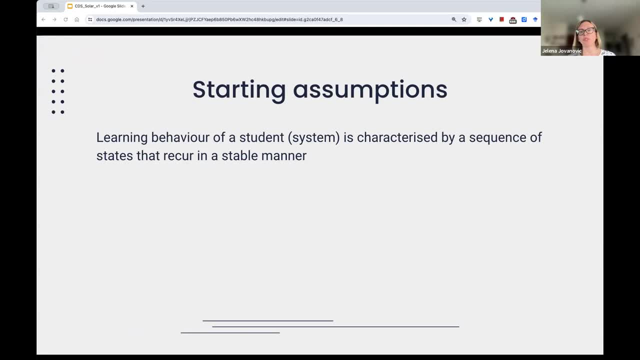 I haven't seen my screen OK, so of course, by drawing on the CDS theory. we started with the assumption that a system that is student, in our case, generally exhibits stable behavioral patterns, that is, stable recurrence of learning states. 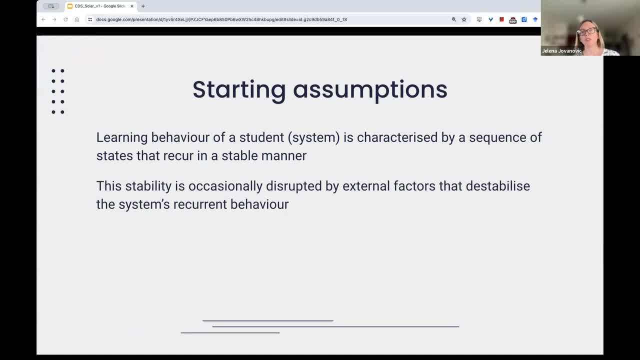 However, this stability in behavioral patterns is occasionally disrupted, And it is typically disrupted by external factors that tend to lead to increased variability in the system's behavior, And such a disruption or destabilization can indicate a phase transition. so the one that Sasha was talking about associated. 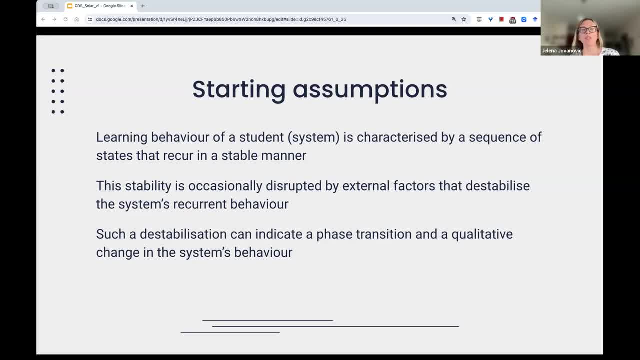 to a qualitative change in the system's behavior. In other words, if a student switches from a more orderly to a less orderly behavior, we can expect that the qualitative change in behavior will take place, Or, in CDS terms, the system transitions to another phase. 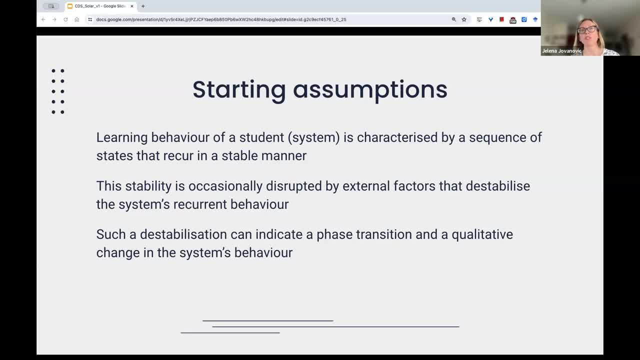 For example, in cognitive science research, it has been demonstrated that, in the context of cognitive development, such a disruption can move a learner from one developmental phase, such as not being able to solve a problem, to another developmental phase, such as being able to find a solution. 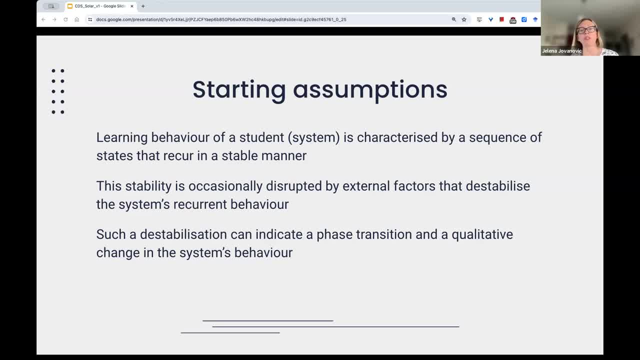 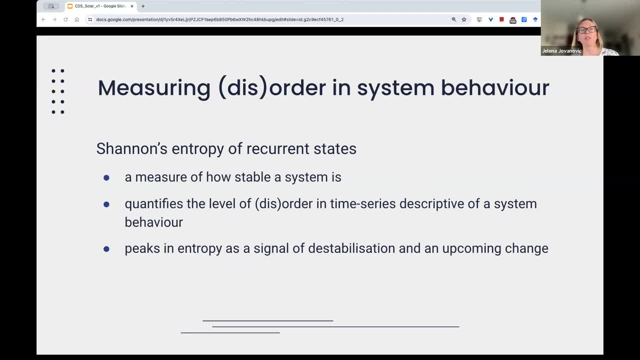 And then the question is how to identify changes in the level of orderliness, So in the system behavior, that is, how to identify these phase transitions, And one option is to do so is to use Shannon entropy, which has actually been widely used to estimate. 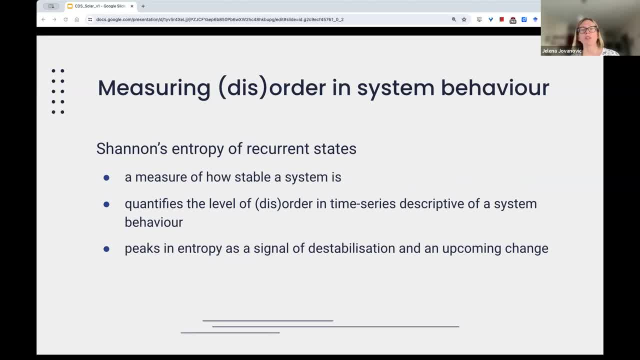 how stable a system is. More precisely, Shannon's entropy has been used to quantify the level of disorder in time series descriptive of a system behavior. And peaks in entropy will reflect the destabilization of the current state and the signal and upcoming change. And with those starting assumptions, 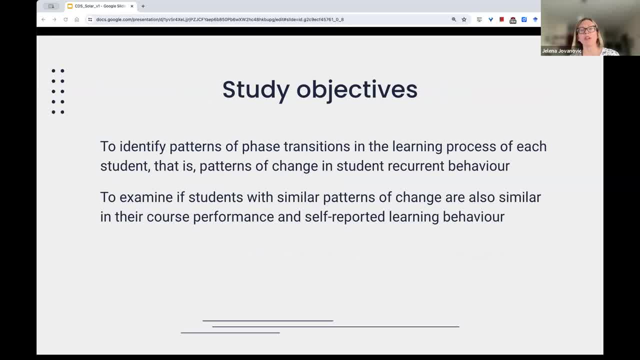 we said, the following study objectives: First, we wanted to identify patterns of phase transitions in the learning process of each student, That is, to identify patterns of change in student-recurrent behavior within a course. And then we also wanted to examine if students with similar patterns of change. 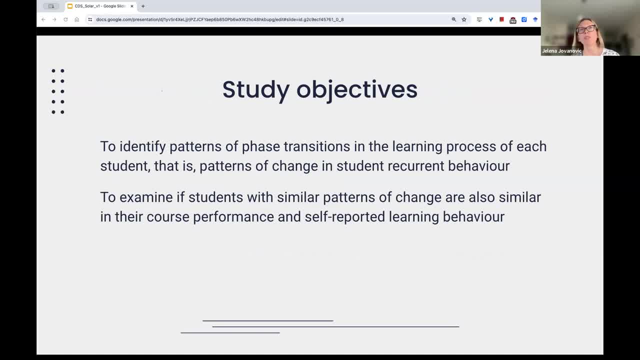 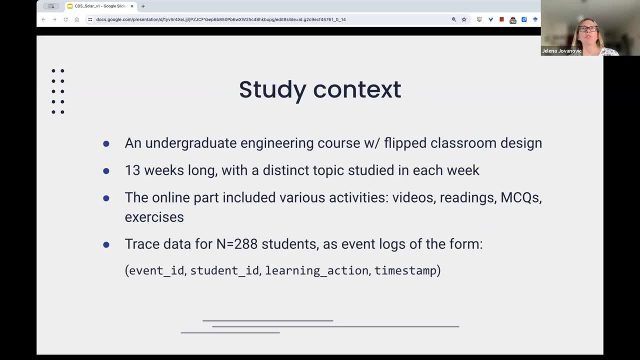 in other words, with similar dynamics. indicators are also similar In terms of their course performance and their self-reported learning behavior. So the study context was an undergraduate engineering course with a flipped classroom design. The course was 13 weeks long and it. 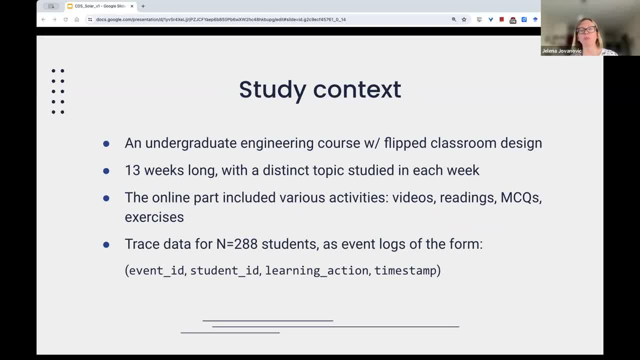 had a weekly structure, in the sense that there was a distinct topic studied in each week And, as I said, it had this flipped classroom, let's say design, where the online part of the course included various kinds of learning activities that were available to students. 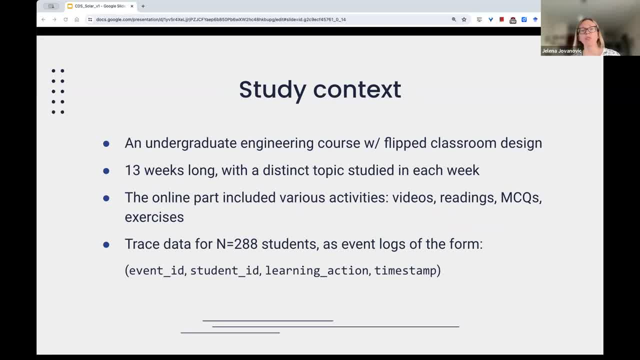 to prepare for the face-to-face part of the course And those included watching videos, reading course materials, doing multiple choice quizzes, which served as formative assessment, or doing exercises, which served as summative assessment, And we had the trace data for 288 students. 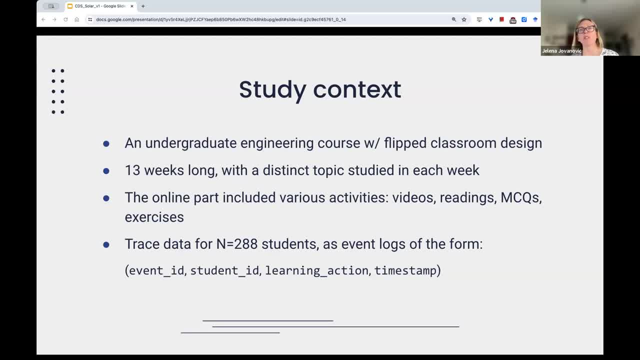 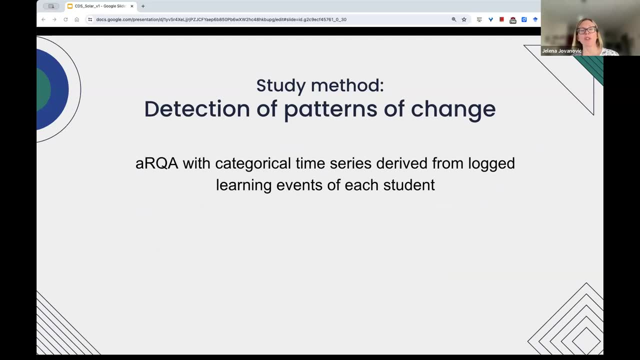 And, after some cleaning and transformation, we actually had the event logs of the format given here. So event ID, student ID, learning action or learning action is one of these that I have just mentioned, and the timestamp And regarding the study method for our first objective. 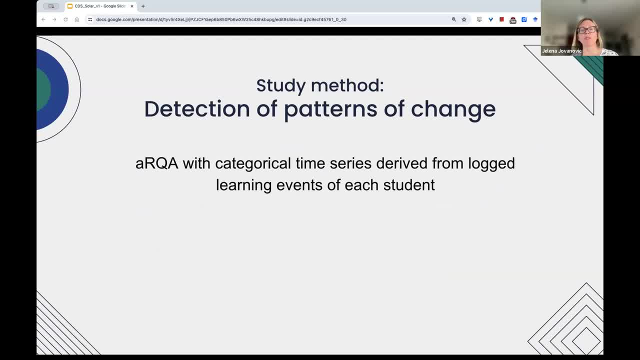 namely to identify patterns of change in student-recurrent behavior. we used ARQA- that is, auto-RQA that Liz talked about- with categorical time series that were derived from log learning events, And I will explain in a moment how we did that. 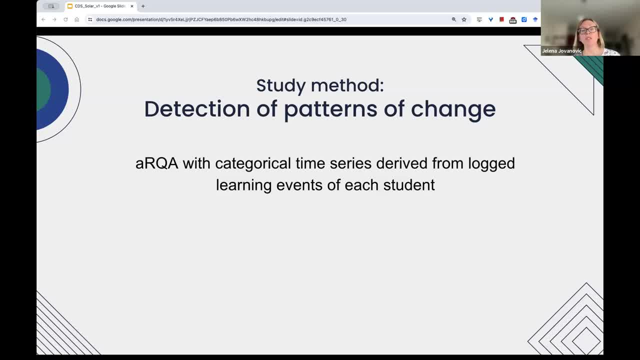 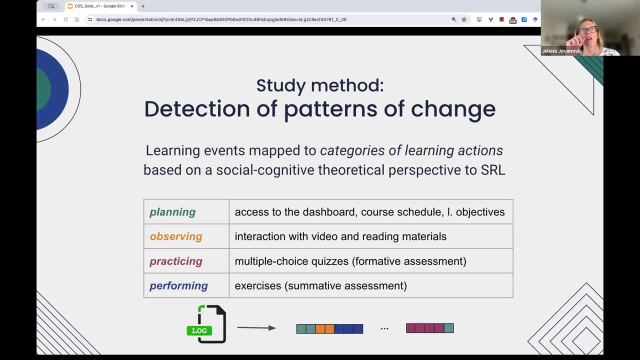 And we did this ARQA For each student individually and for each week of the course. That is, for each student and each week of the course. So, regarding this time series, that was required for ARQA, so we mapped actually a lot of learning events. 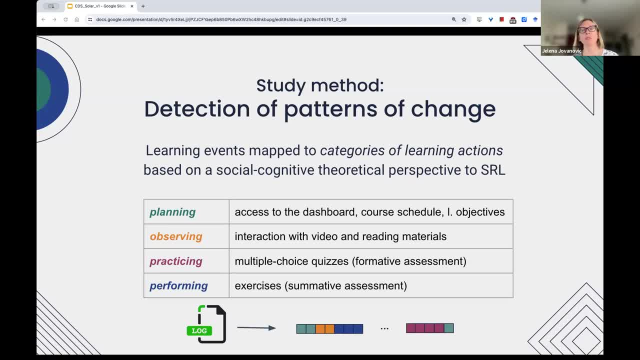 into course-grained categories of learning actions that correspond to different types of SRL behavior. More specifically, we adopted a social, cognitive theoretical perspective to SRL- Self-regulated learning- with an understanding that the student goes through a sequence of learning behaviors that is, in CDS terminology, learning states which 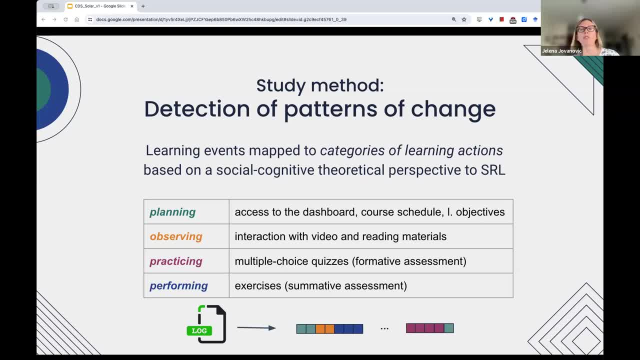 include observing something in a social pane through video readings, internalizing it through practicing and evaluating the effectiveness through performing and adapting it And accordingly, we recorded learning events, that is, actions in learning events, into four categories: Planning, observing, practicing and performing. 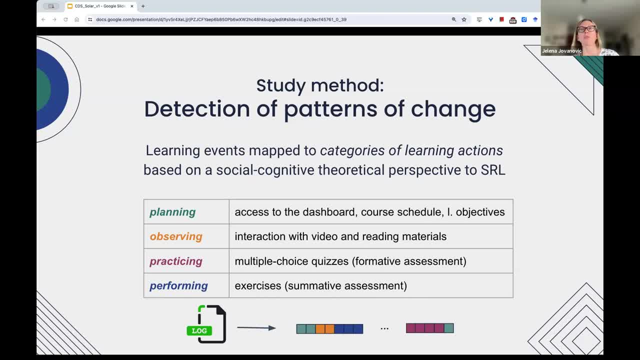 So planning was everything related to the access to the course schedule and to the learning objectives, which are available for each week of the course, And also to the dashboard that was available to students for reflection. Then observing was everything related to the interaction with the video and reading materials. 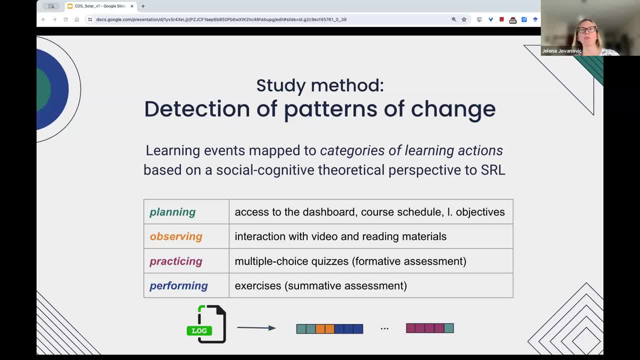 Practicing was about interaction in multiple choice quizzes as a form of formative assessment, And performing was about interaction with exercises, which primarily served as summative assessment, And in that way we actually mapped logged the events into this kind of sequence of these four categories. 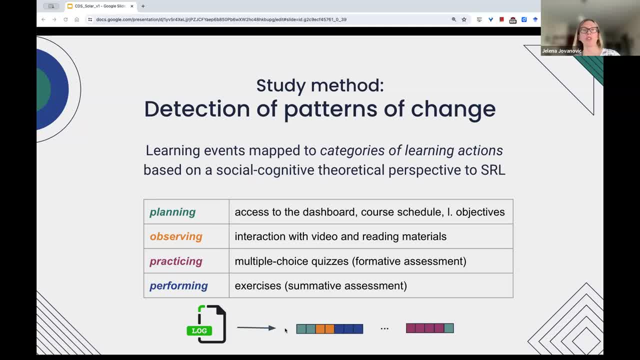 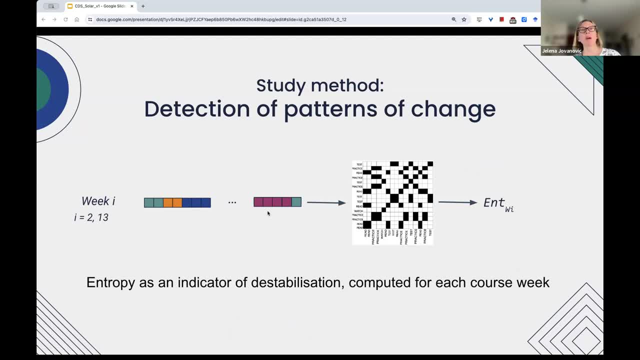 of learning actions, And this was done, as I said, for each student and for each course week. So, having done this mapping, then we use this kind of categorical time series as the input to ARQA and got a recurrence plot as the output. 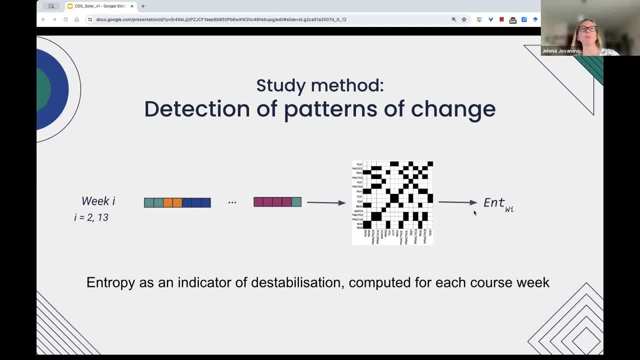 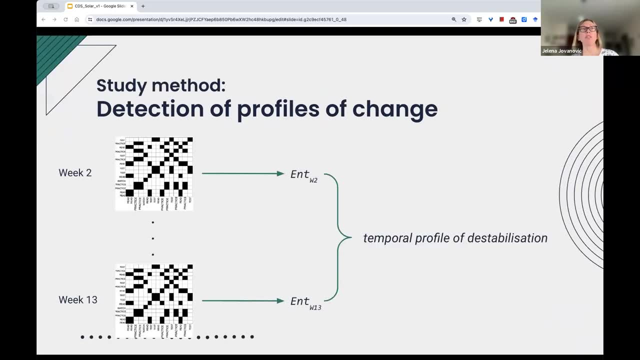 And then, based on the recurrence plot, we computed entropy as an indicator of destabilization. Regarding the recurrence plot, we do not have time to explain it here, But in the paper you can take, a nice explanation is given. And then, regarding the second research objective, 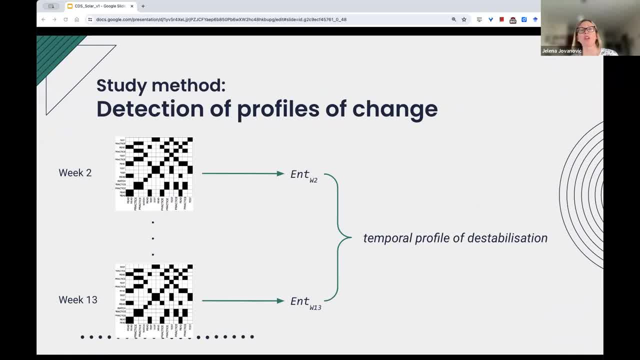 so the detection of profiles. So we started from these computations of entropy for each student and each week And in that way for each student we got a kind of sequence of entropy values for the 12 weeks, So from week two to week 13,. we didn't do it for the week one. 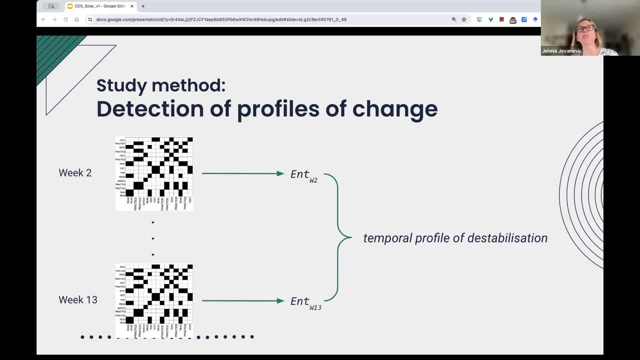 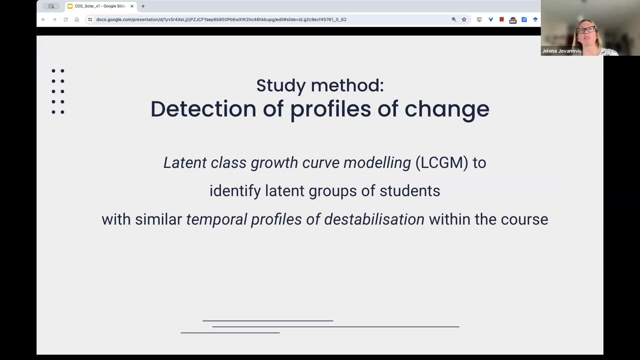 because that was the preparatory week for the course and no real learning was happening. So in that way we got a temporal profile of destabilization For each student and starting from that we actually did a kind of clustering of students using a method which is called latent class growth curve. 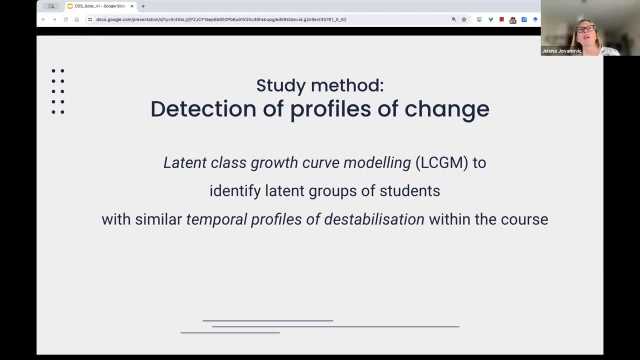 modeling, or LCGM for short, which actually combines latent class analysis and growth curve modeling, in the sense that for each student, we first estimate a growth curve based on the measurements of entropy values for individual weeks, And then we cluster students based on the estimated growth. 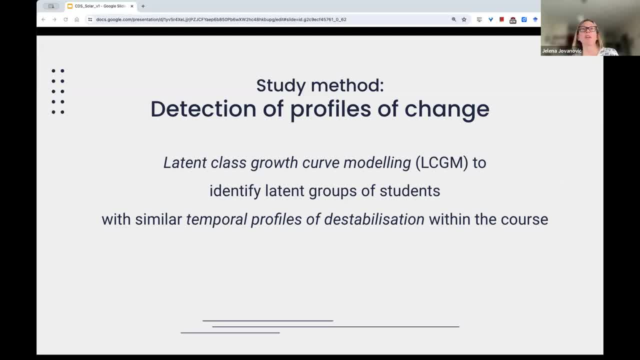 curve parameters And in that way we actually managed to identify latent groups of students with similar temporal profiles of destabilization in the course, And we did this LCGM for different numbers of classes or clusters and got the best model for three classes. 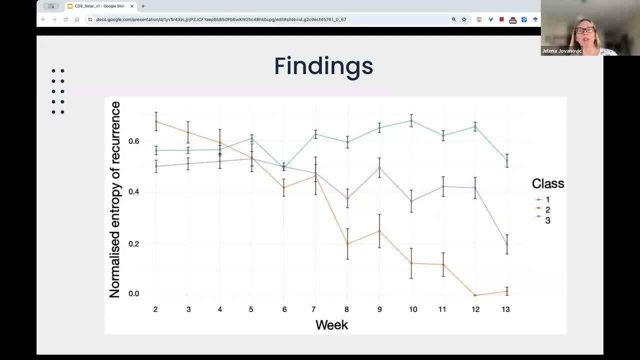 And this is the one that we used. And we did the LCGM for different numbers of classes or clusters and got the best model for three classes And this is the one that we used. And this is the one that we used. This is the one that we kept and further analyzed. 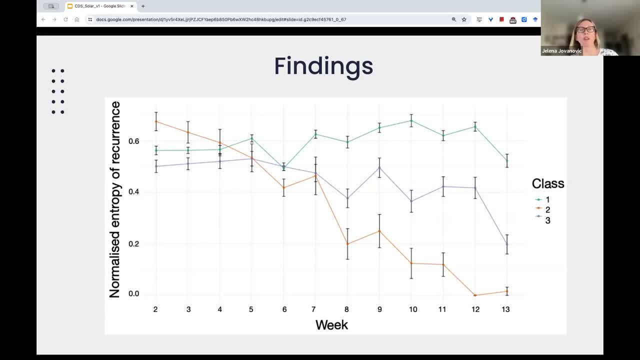 To do this analysis and interpretation of the profiles, we started from this plot. This is a plot with the means and standard errors of weekly entropy measures for each latent class or each profile. It says here: normalized entropy. Normalized means just that it's in the scope of one range of 0. 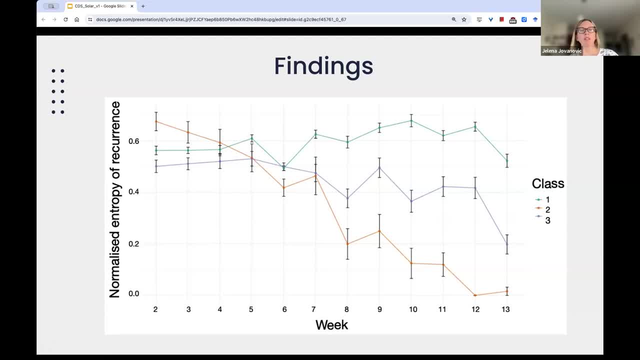 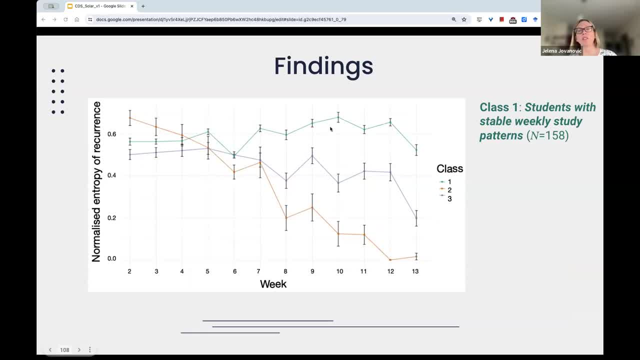 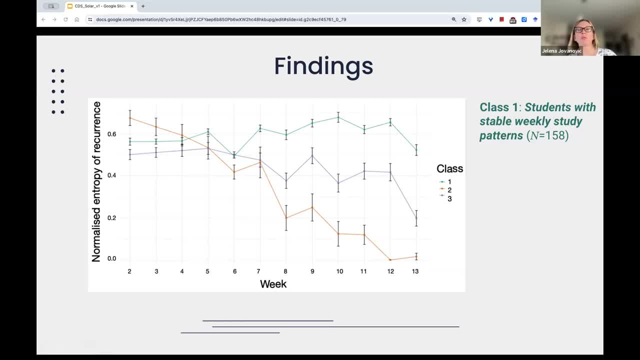 with 158 students, It gathers students whose entropy of divergence weekly activities remain fairly stable and relatively high throughout. The only drops happened in week 6 and week 14, which where the weeks of mid-term and final exams. 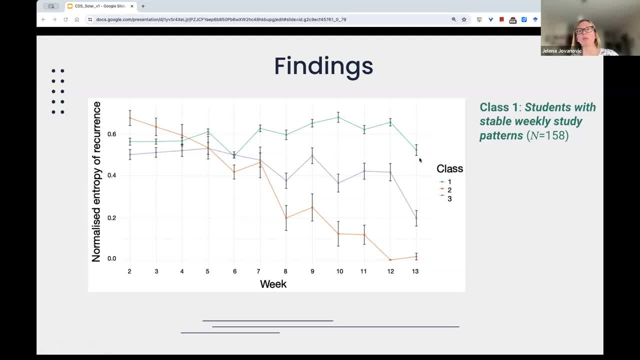 And we assume that the intensity proportions was very high. Preparation for the exam actually reduced the variability of behavior to exercises and quizzes- actually not assumed just, but checked it in the data. The second profile is about students with steep changes in weekly study patterns. 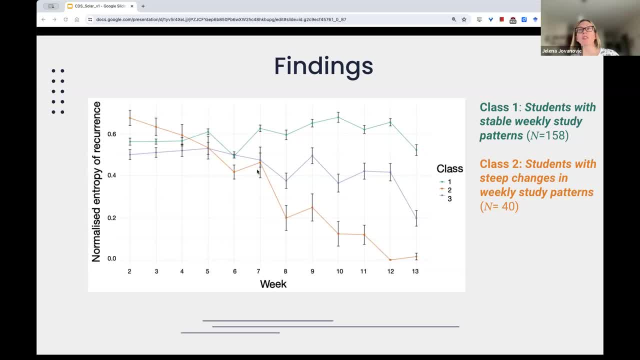 So this is the orange one and this is the smallest profile, with 40 students, And we can see that this is the profile that starts with the highest entropy values. but already from the very beginning those entropy values start going down and steadily go down, with some significant drops, especially between week seven and eight. 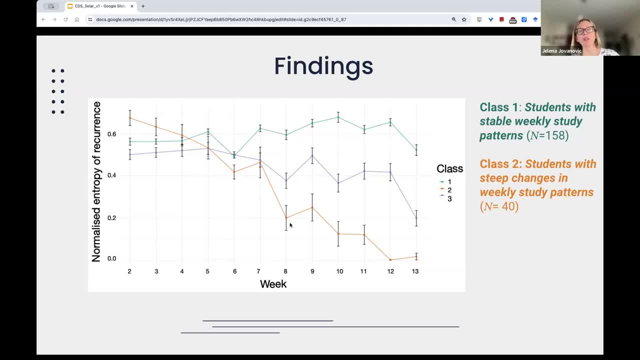 And we assume that these are students who continuously and occasionally significantly change their behavior towards the last diverse ones. And also, this Profile actually exhibited the- I mean showed the lowest exam scores both on midterm and final exams and significantly lower compared to the other two profiles. 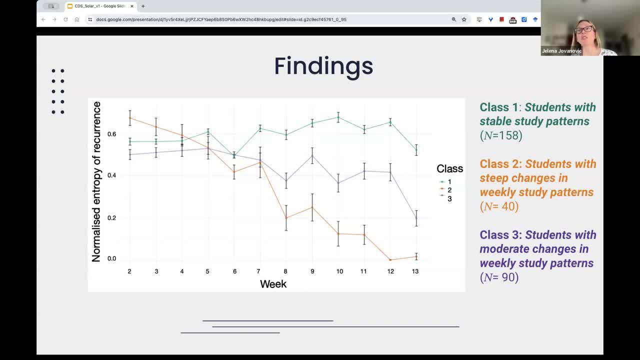 And the third profile includes students with moderate changes in weekly study patterns. So those are the students who started. so the violet one, So students could start with lowest entropy. that is, high stability of recurrence in behavior, And experienced slight decrease throughout the course, only with the significant decrease towards the very end of the course. 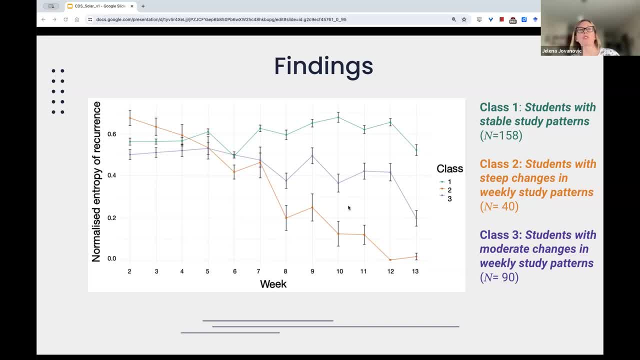 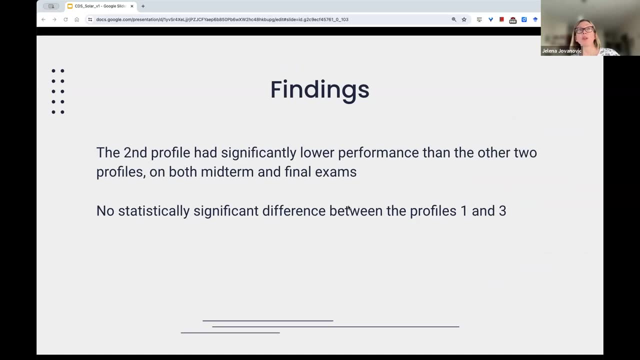 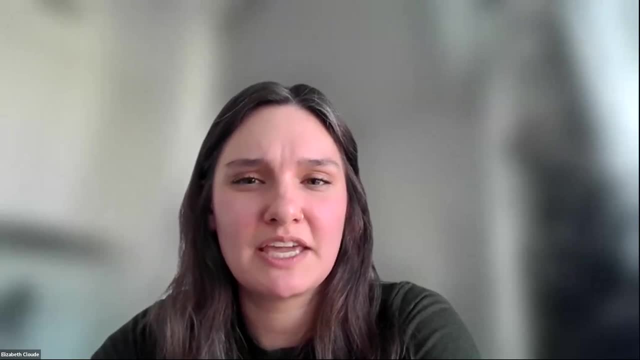 Whereas the second profile has significantly lower performance compared to the other two, both midterm and final exams. We're actually doing a bit with game mechanics, So different kinds of game mechanics which are designed to elicit different emotions in a future study. But thank you for that. 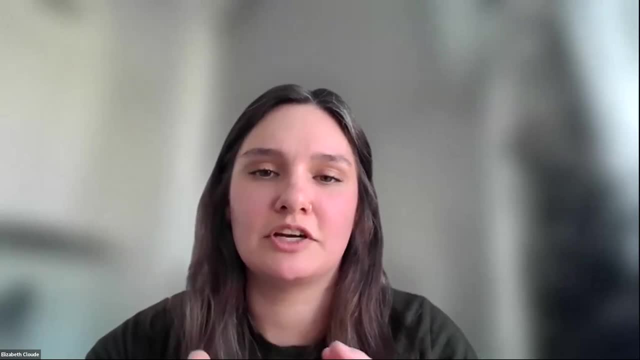 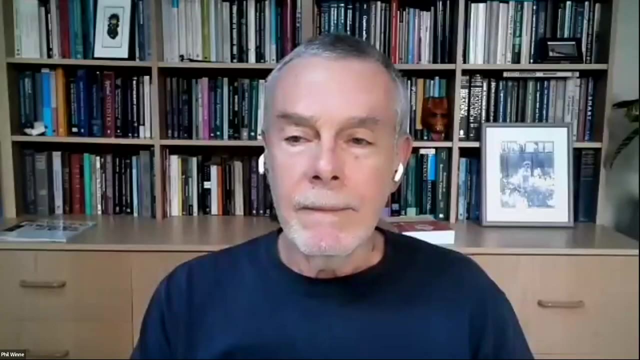 That would be interesting to include potentially in the different variables that we're modeling here, because that could provide insight into cognitive appraisals. for example, that dimension, Yeah, and get it that aspect, Picking out that model, it's the cognitive appraisal that leads to everything else. 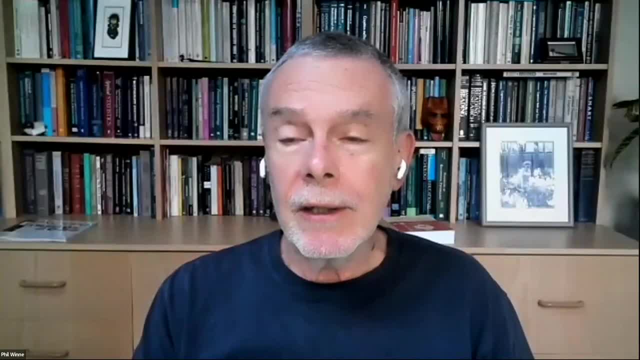 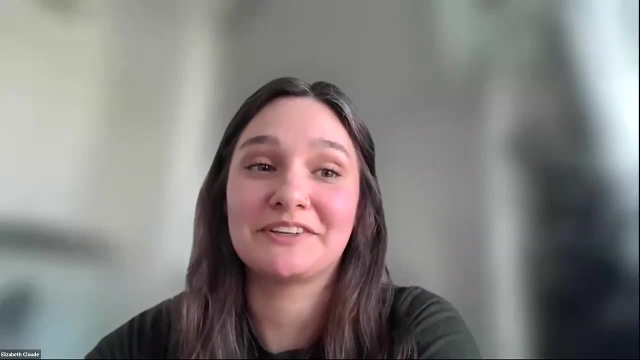 And to identify what the appraisal is. it might be helpful to know what the information in the presentation at the point in time is as a differential compared to the prior knowledge the person has. That's very granular, that part, Absolutely. Sasha had a point. 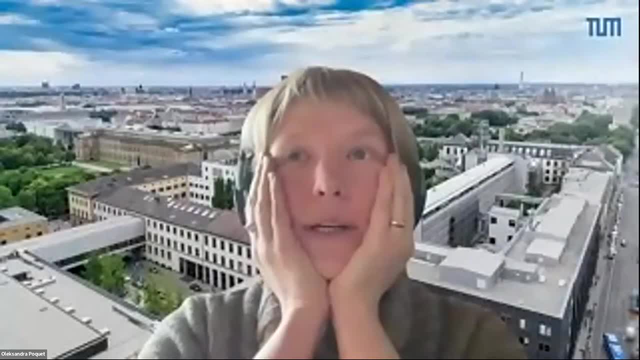 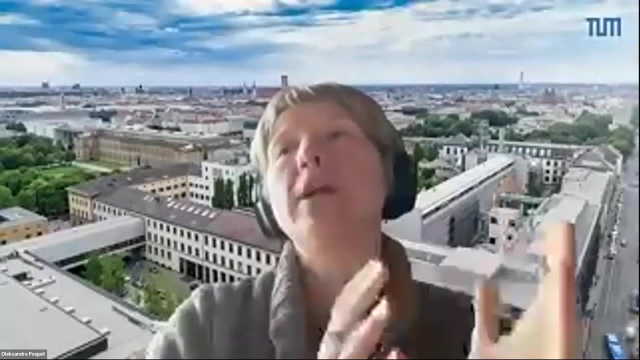 Yes, I wanted to add quickly that I think that that's key, but it's key for asking a lot of questions that are not the kinds that we framed in the beginning, right, So you can ask two sets of questions, or at least that's my understanding of it. 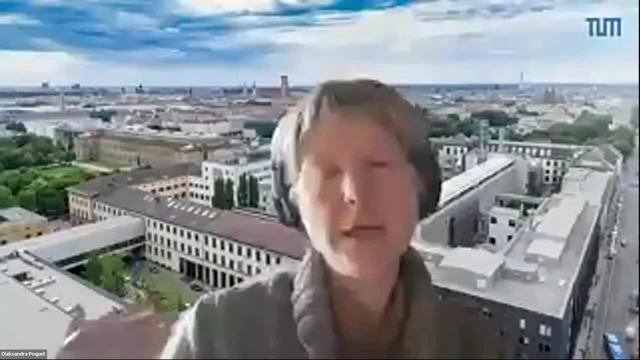 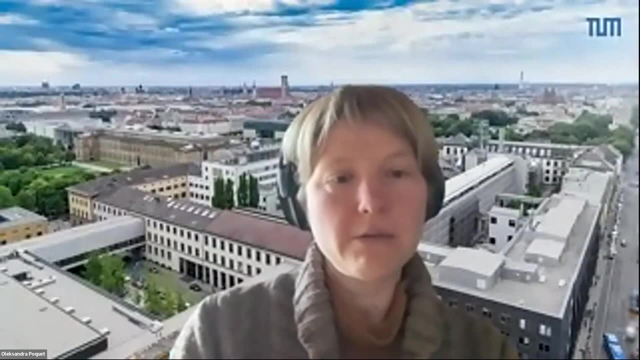 We can start asking: is there a pattern to the process and what's that pattern? And then we can start asking why we're observing the pattern we're observing And, theoretically speaking, determining a pattern does not require the right variable, because we can still understand the dynamics of what's happening and start looking for. 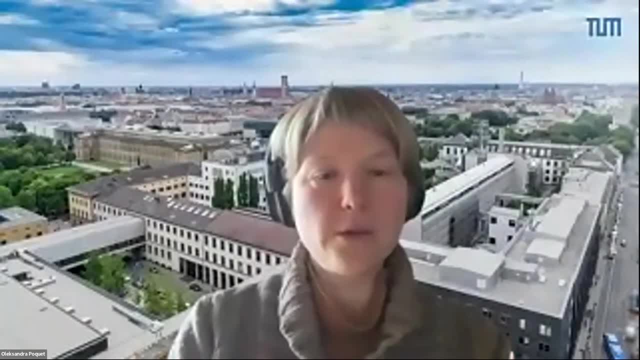 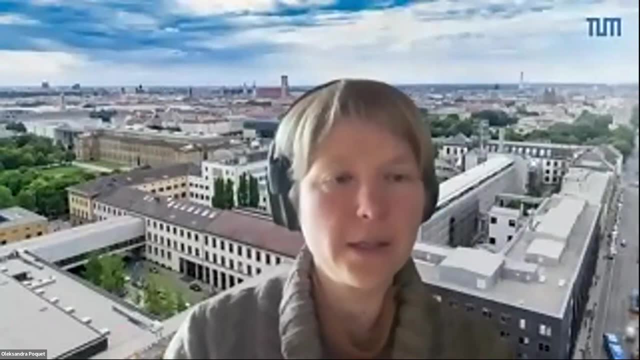 things. However, if we want to start understanding sort of relationships between the different processes, Then we have to go back to the theory, And that's also what we've discussed with Jelena, that in our example, obviously, if it's building on theory that uses information processing and it's not in the picture, we 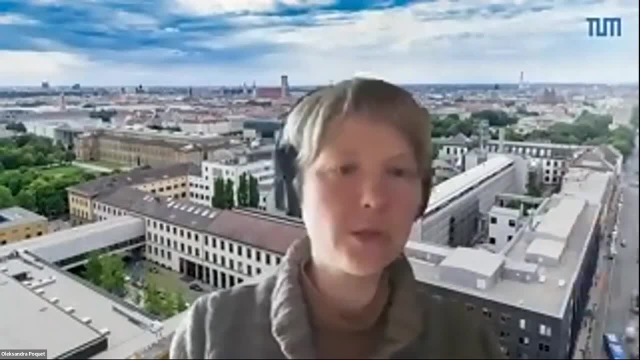 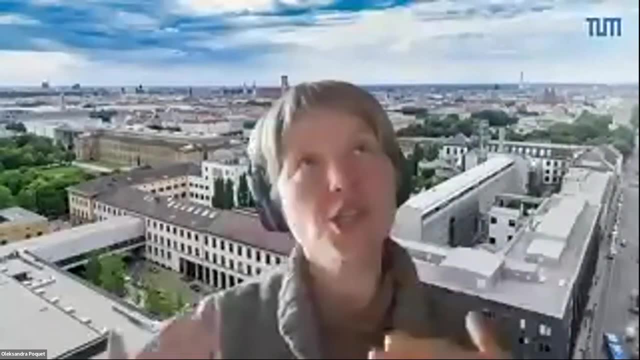 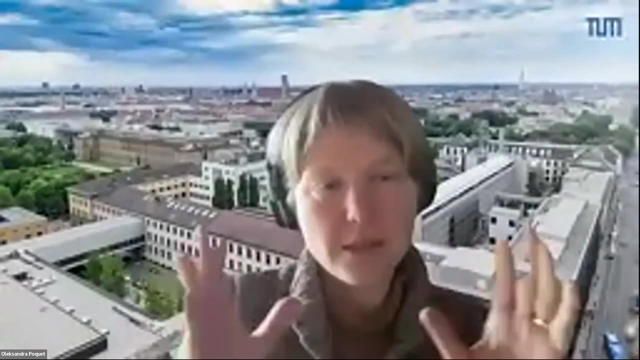 cannot explain what we're seeing, because it's just not there. And, yes, I think what you're suggesting, even looking at that in relation to behavior, might make some suggestions as to what's happening. But again, RQA itself, in my view, without, as it's presented, been presenting in the 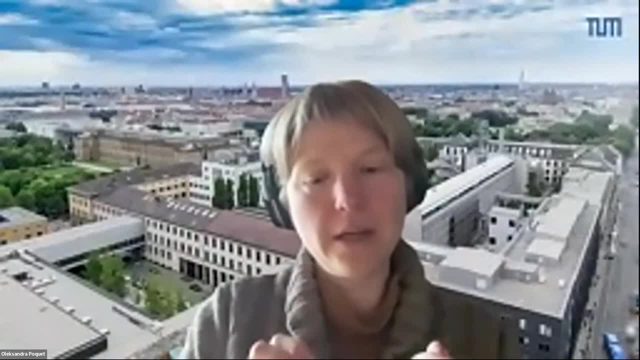 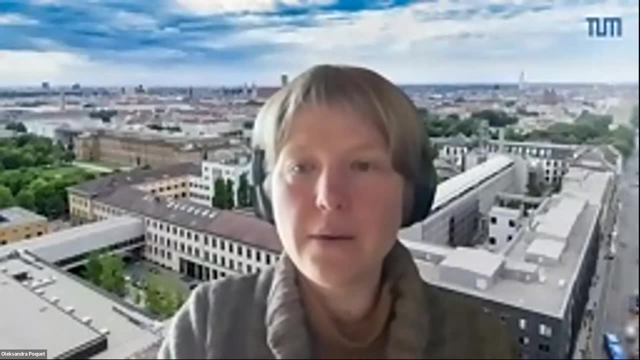 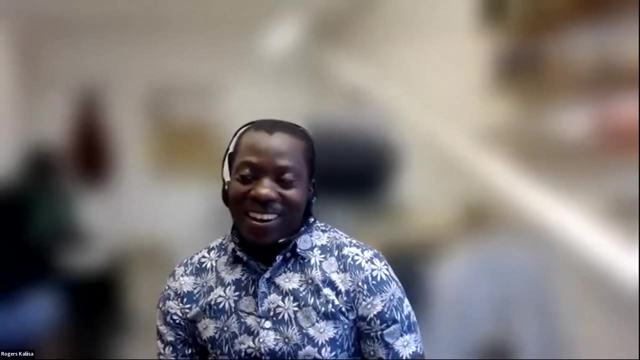 studies will always only tell us about the pattern rather than a little bit more. We need to do a little bit more with that, to start asking the kind of questions that explain things. Sorry, sorry, sorry, I thought you had finished. Okay, I think we have. we had more questions in the chat. 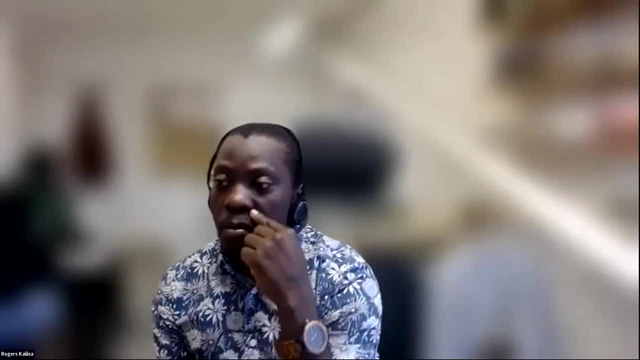 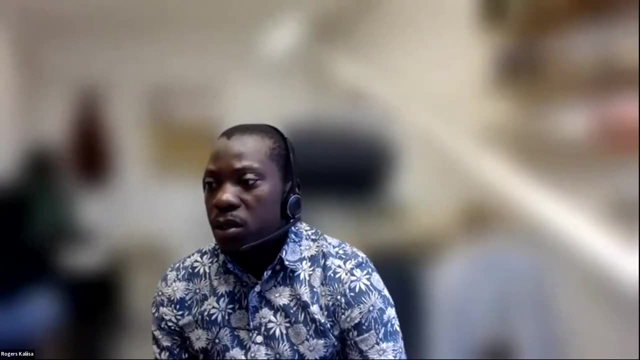 I think you can see. Joel was asking whether emotions could vary based on age, which could be similar, like what happens in marketing Marketing applications, and as to whether it would be interesting to see if there are differences in emotionally provocative course content versus more dry course content. 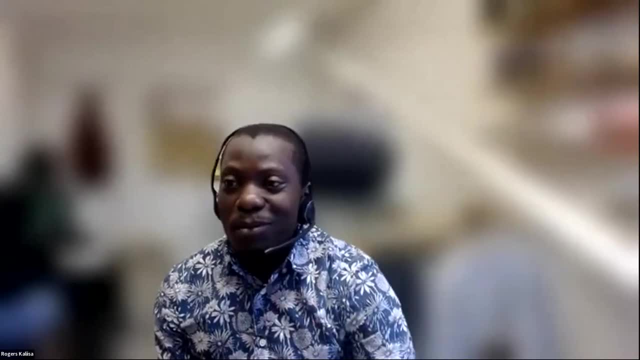 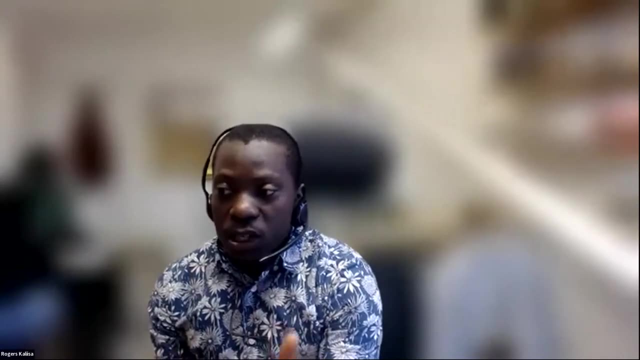 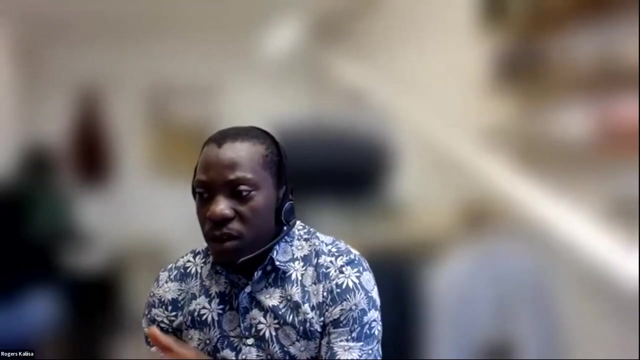 For example, if you're teaching science or biology, maybe students are emotionally more like provocative than teaching very serious things, And so whether that could actually change. So that's about disciplinary content and how that varies with emotions And whether it's the same, whether it varies between content.